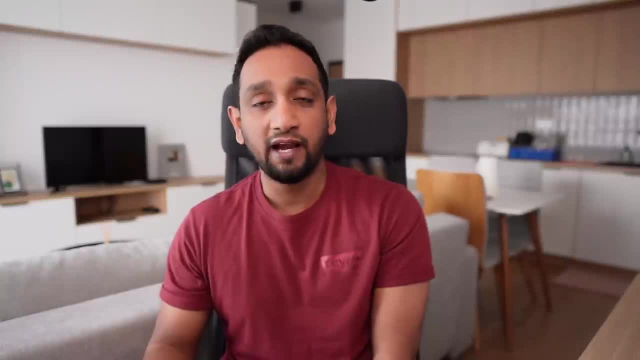 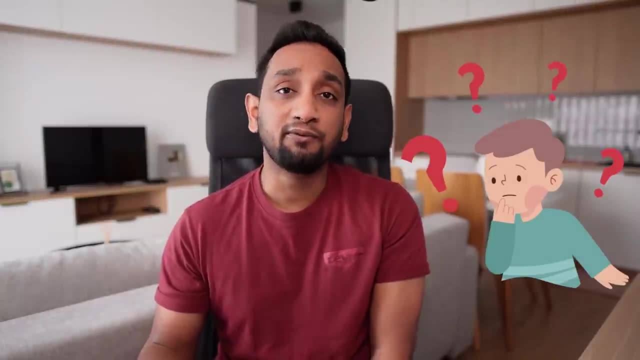 Hey everyone, I know a lot of you guys are looking to learn SQL and I know that you prefer to learn SQL for free, but the challenging part is: how do you get started and, more importantly, what are the different concepts you will need to learn, based on your requirement? right, Because there are so. 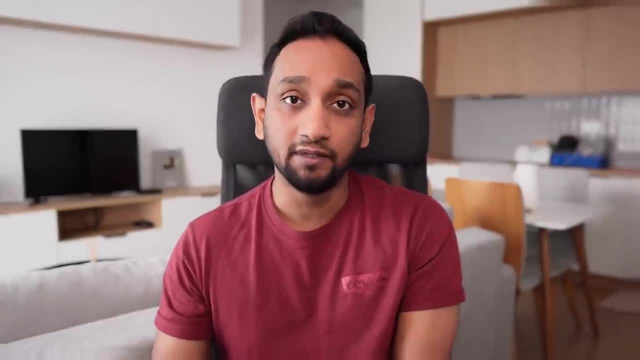 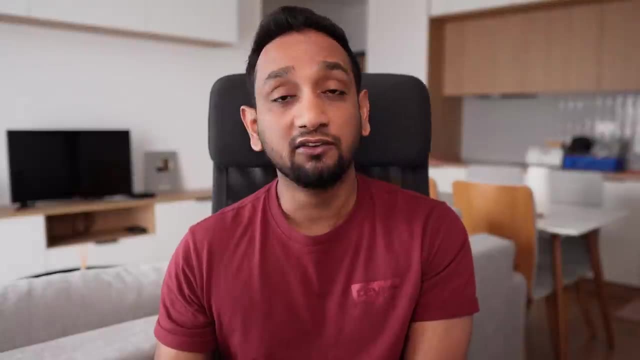 many different concepts in SQL, so do you need to learn each and everything? Different jobs would need a different level of SQL expertise, so some of you guys might just want to learn basic SQL. some of you guys might be looking to learn intermediate level of SQL. there might be. 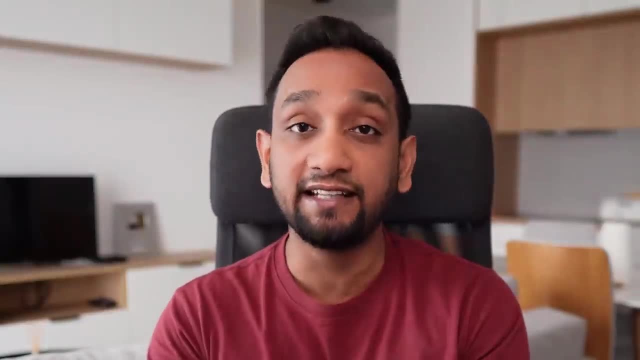 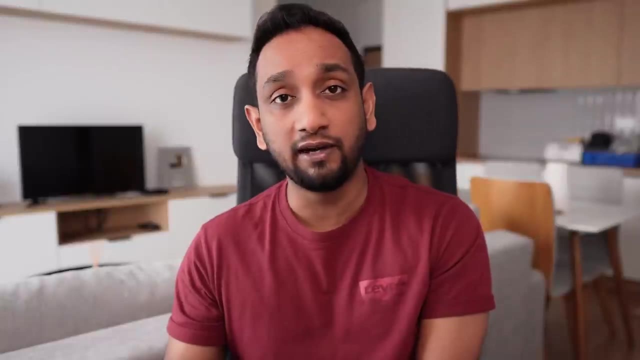 others who already know the basics and intermediate, or at least they think that they know, and they would want to learn advanced SQL. and there are others who are looking to become a database developer or an SQL developer. In that case just the normal SQL would not suffice. You might want. 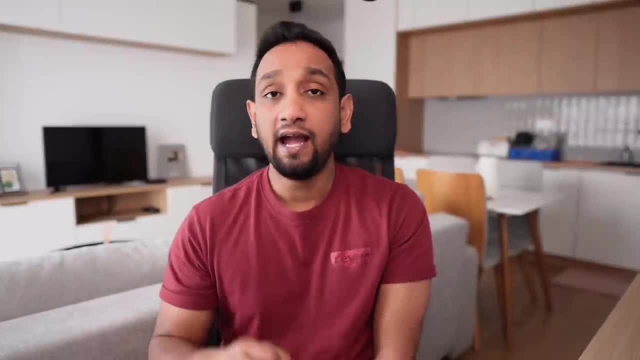 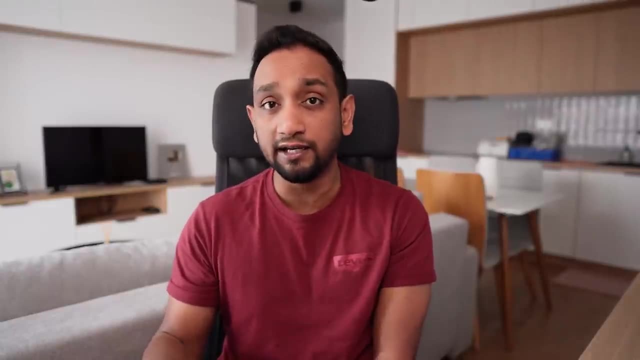 to learn certain additional SQL concepts right, And that is why I wanted to make this video a complete SQL roadmap, where I'm going to mention all the different SQL concepts you will need to learn, based on your requirement. So let's get started. 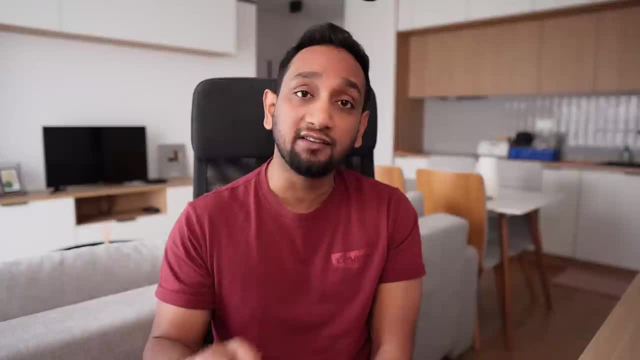 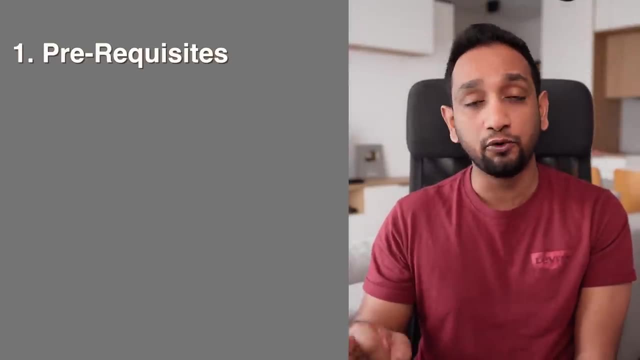 Based on the level of expertise you want to gain in SQL, based on your job or whatever you are looking for. So I have divided this video into five parts. In the first part, I'm going to talk about all the prerequisites: how do you choose a database, what tools you need, etc. The next four 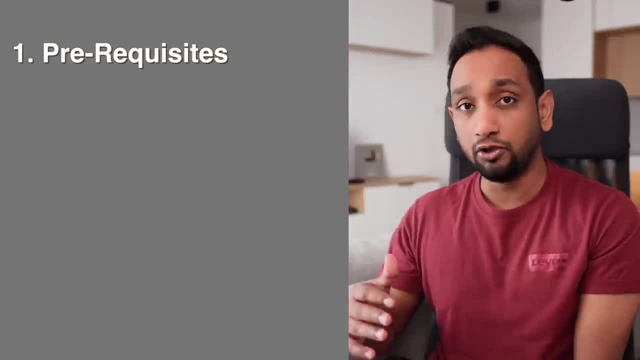 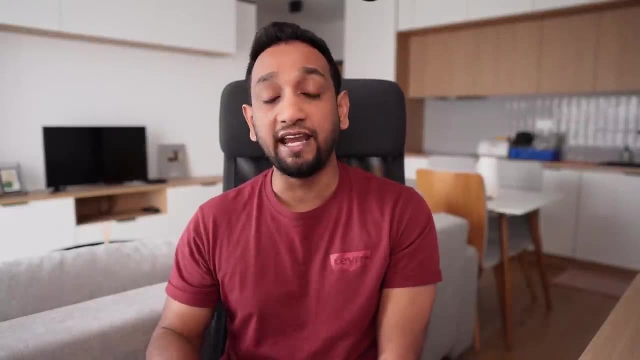 parts. I'm going to split them based on the level of expertise, So I'm going to have a basic, intermediate level, advanced level and SQL for developers. Under each of these sections, I'm going to mention exactly what SQL concepts you will need to learn. I'm also 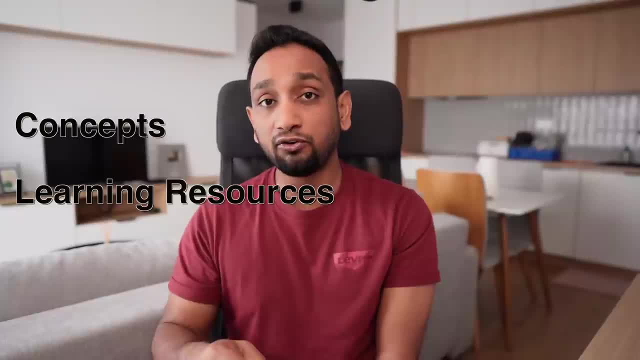 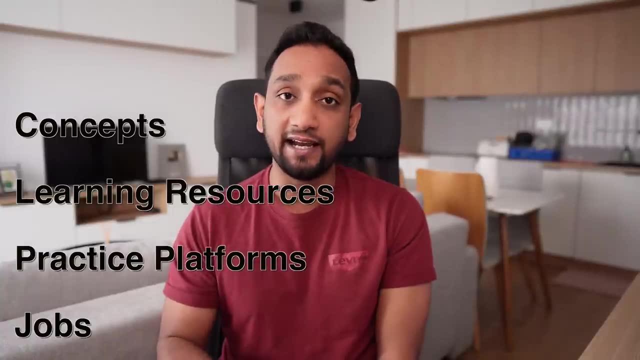 going to mention the resources that you can use to learn these concepts, And I'm also going to mention the platforms that you can use to practice these concepts And, of course, I'm also going to mention the jobs that you can target under each of these sections. Now, before I can start the 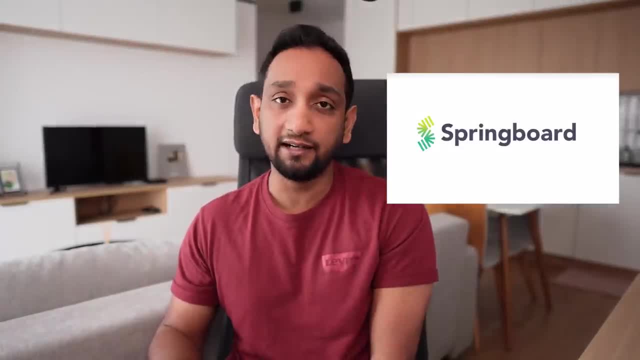 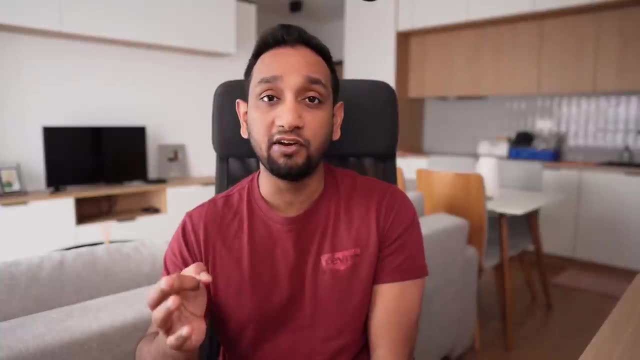 video is sponsored by Springboard. I'll talk more about them a little later in the video. So let's start with the prerequisites Now. the very first thing that you need to understand is: SQL is basically a programming language that is used to interact with relational database, right? So 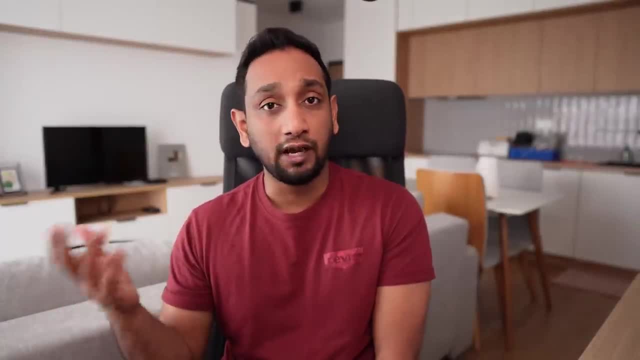 let's say you are building an application. So let's say you are building an application. So let's say you are building an application or a software. Now your application would definitely need data, right, But the data is generally not stored in the application itself In most cases. 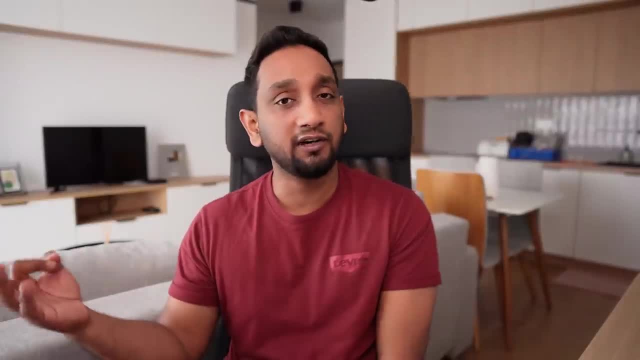 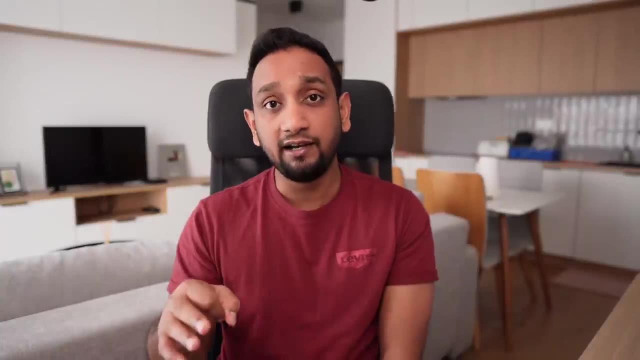 the data is stored in a relational database right Now. of course, there are non-relational database as well, which does not need to use SQL. I'm not talking about them. I'm only talking about relational database, And currently the most widely used database is still relational. 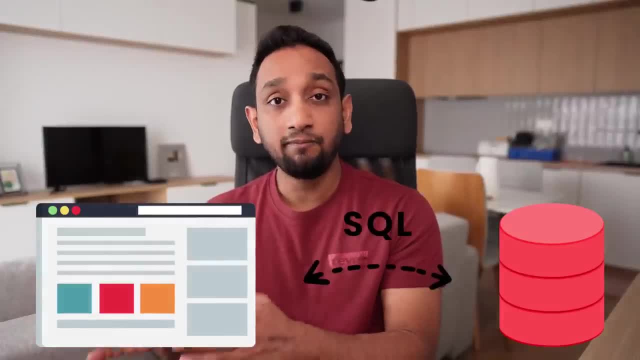 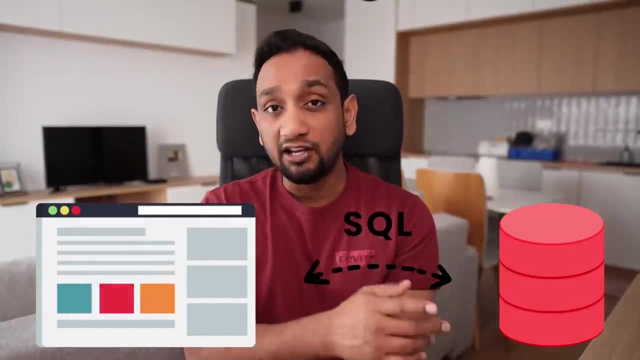 database. okay, So you have an application. It needs data. The data is stored in a relational database, So there needs to be a way for your application to interact with the application. So relational database only understands one language, and that one language is SQL. So 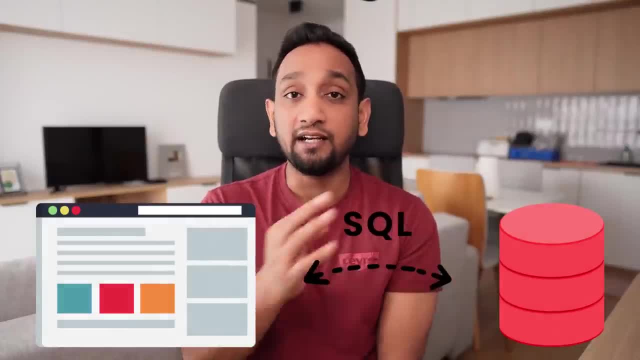 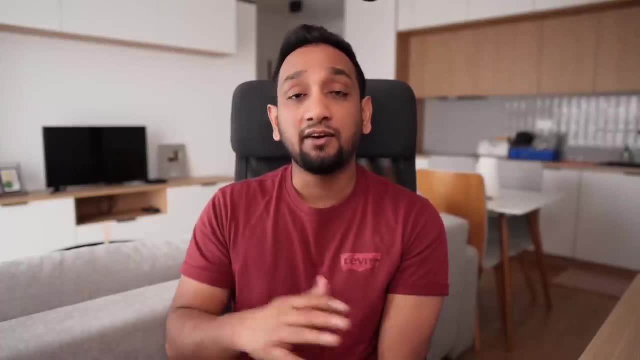 if your application needs to communicate with the relational database, then it has to communicate in the language of SQL only, and that is why you need SQL. okay, Now the problem is there are several different types of relational database. Now the most popular relational database as of 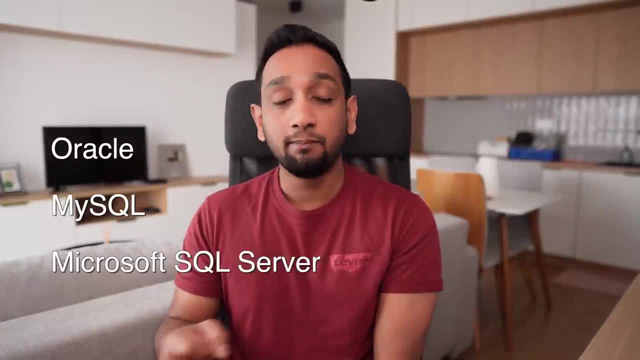 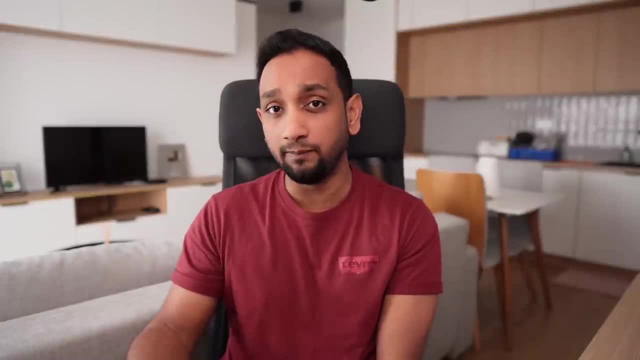 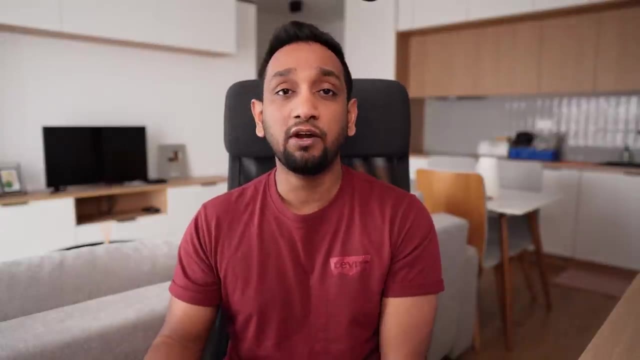 December 2022 is Oracle, MySQL, Microsoft SQL Server and PostgreSQL. Of course, there are other cloud-based database or data warehouses as well, like Google, BigQuery, Amazon, Redshift, Snowflake, etc. So, among all of these databases, which database should you choose when you are getting? 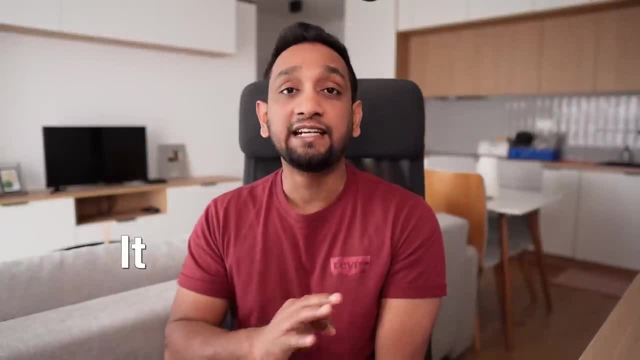 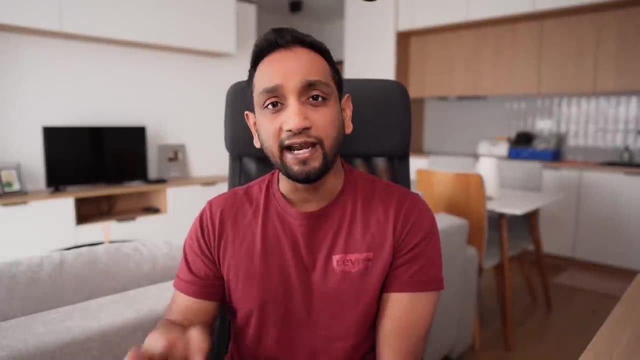 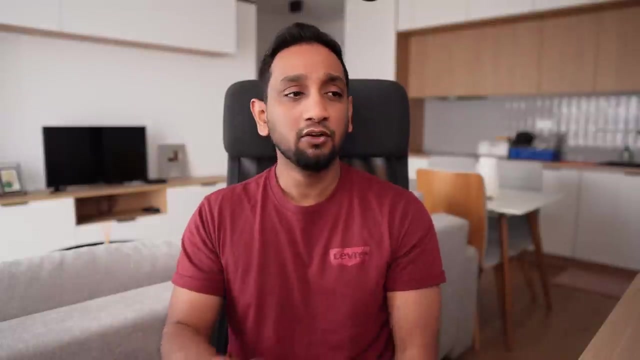 started in learning SQL. A simple answer is: it does not matter, right? It does not matter which database you choose in order to learn SQL, because 80 to 90% of the SQL that is used in all of this RDBMS are basically the same. The syntax is the same, The concepts are the same. So, whatever you, 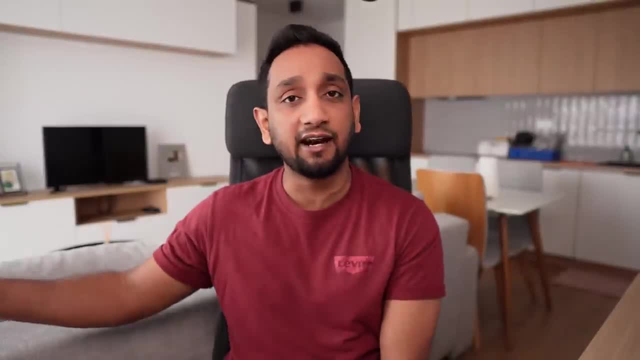 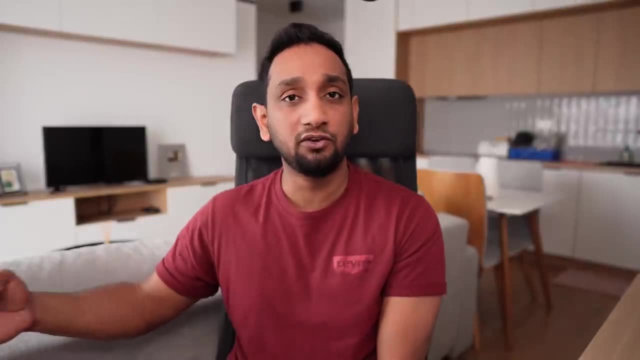 learn in one of these databases, it does not matter. So it does not matter which database you choose in RDBMS. you will be able to apply them in any other RDBMS you might have to use in the future. So let us say you learned SQL in Oracle and tomorrow you get a job where your company is. 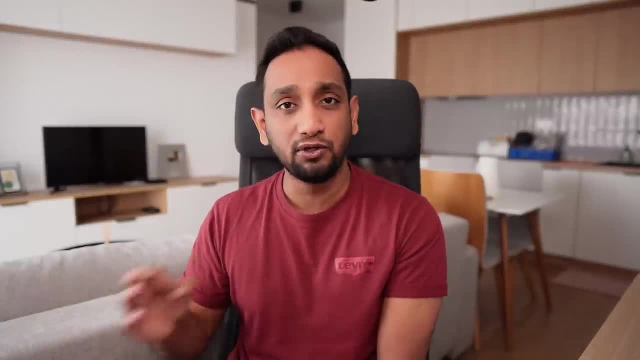 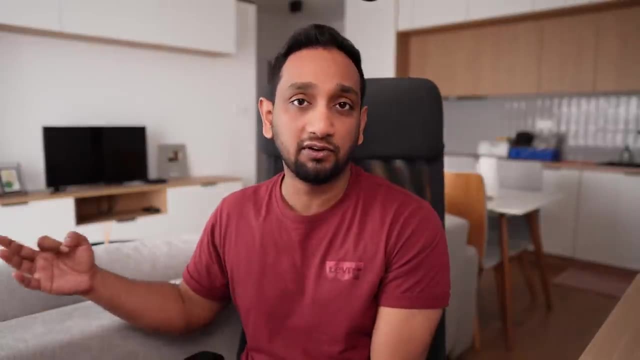 using Microsoft SQL Server. you do not have to worry at all. Within a span of few days you will get hanged on with Microsoft SQL Server and whatever you have learned in Oracle will still be applicable in Microsoft SQL Server. Of course, there might be 10 to 20% of differences. Mainly, 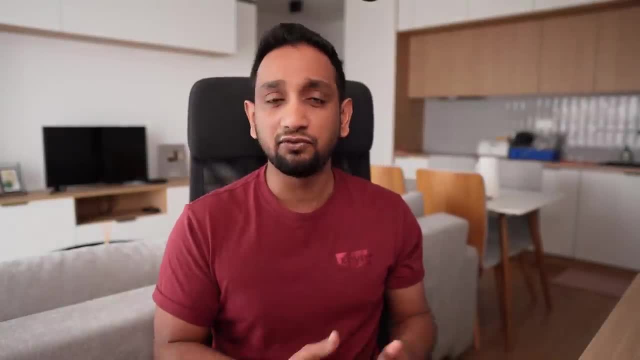 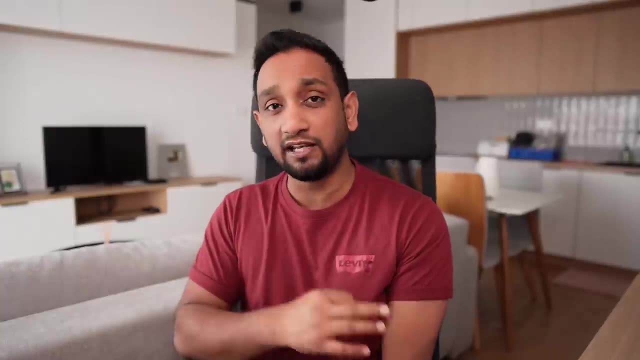 the changes might be in certain functions which like inbuilt functions which might be supported in RDBMS and might not be supported in other RDBMS, But you would generally have an alternate function which basically does the same thing in other RDBMS as well. You just need to Google it. 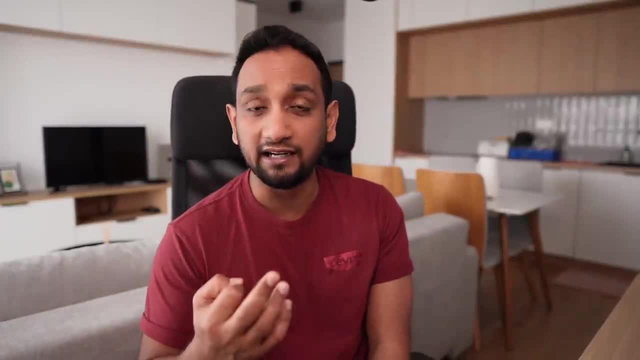 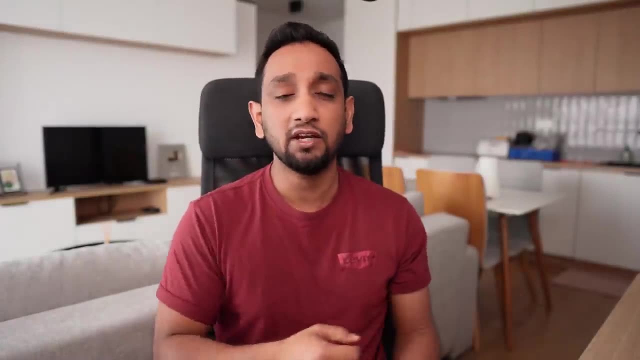 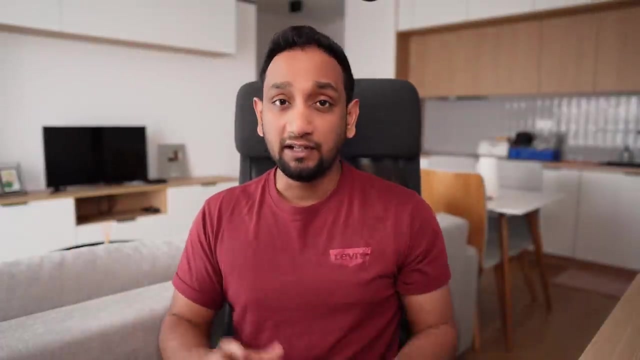 and find those functions. And in some cases there might be some syntactical differences in certain concepts, which would be very minor, which anyone. if you learned a concept in one RDBMS you should be pretty much very easily able to grasp the other small changes in any other RDBMS. So when it comes, 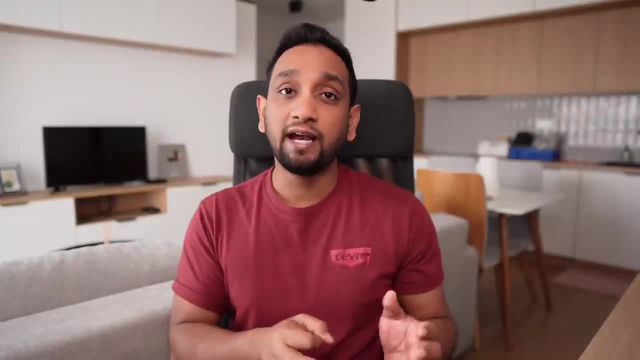 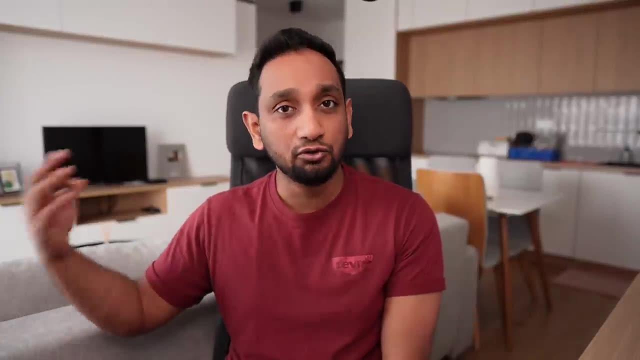 to choosing the RDBMS, it does not matter, But of course you will be able to learn the same thing. if you know that there is a specific RDBMS that is used in your job, or you know that you will be building your project in a particular RDBMS, then it's always better to choose that RDBMS. 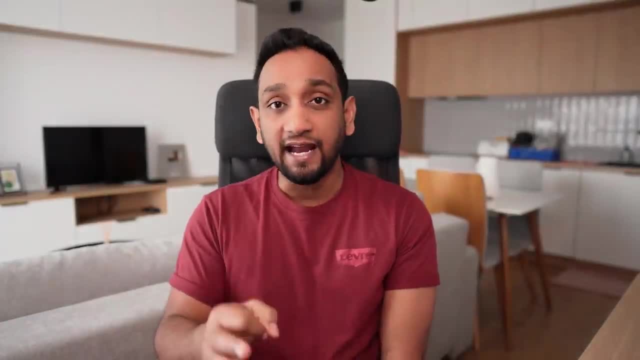 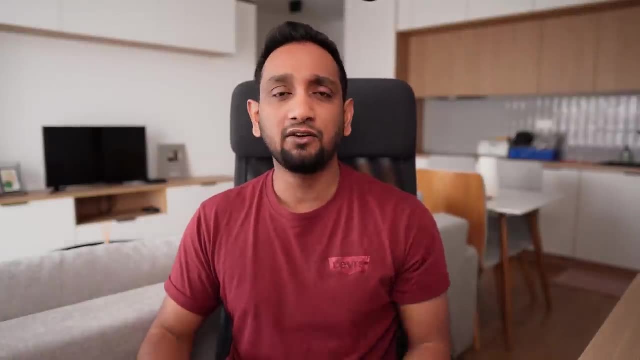 But let's say you do not have a preference. In that case, if you ask me, my personal preference would be to go with PostgreSQL. It's free, it's lightweight and I think it's one of the best databases that you can use, especially if you want to start learning SQL. 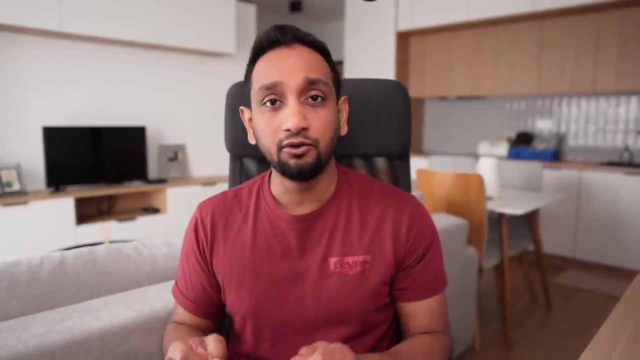 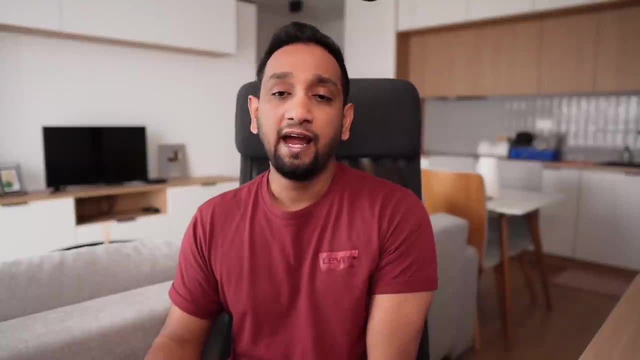 So let's say you have selected your database. The first thing that you need to do is you need to have a database in your system. It's pretty simple. You can install any database of your choice, And if you are using a cloud-based database, then you just need to do a browser. 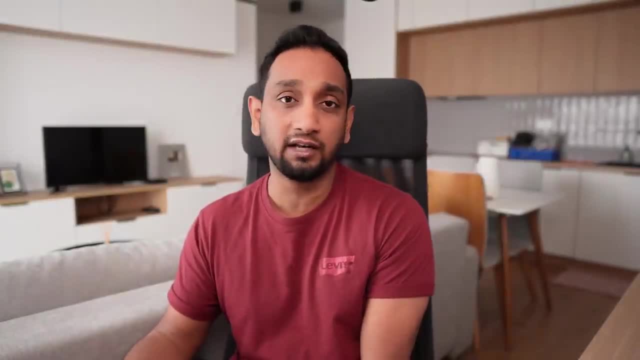 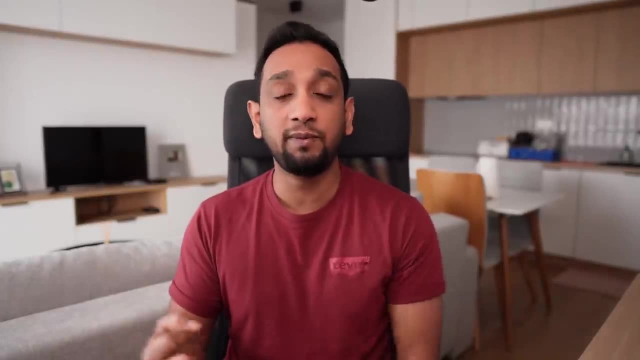 setup, like online setup, of that cloud-based database or data warehouse. And, let's say, once you have installed any of these databases, the next thing is you need an IDE tool with which you will be able to connect to the database and do all the different operations. Now the four. 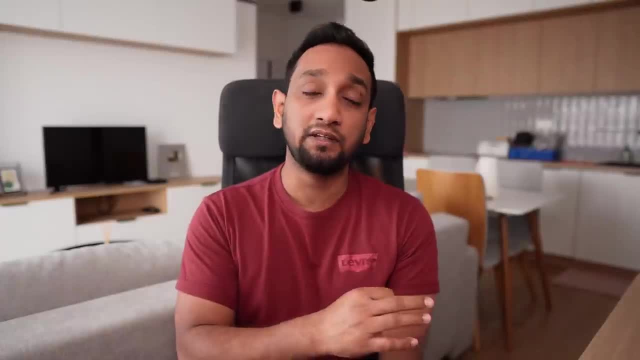 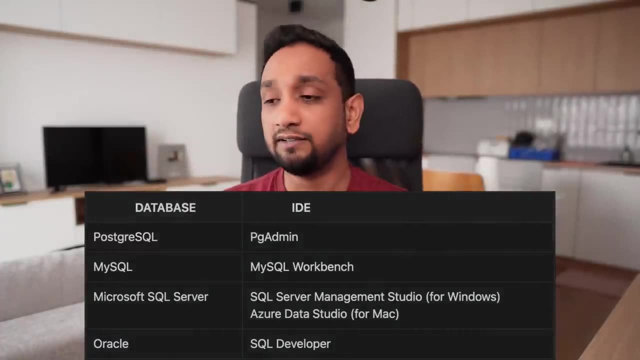 most popular RDBMS I mentioned. each of these RDBMS will come with their own IDE. For example, if you're using Oracle, then it will come with SQL Developer. If you're using Microsoft SQL Server, then it comes with SQL Server Management Studio in Windows, And if you're. 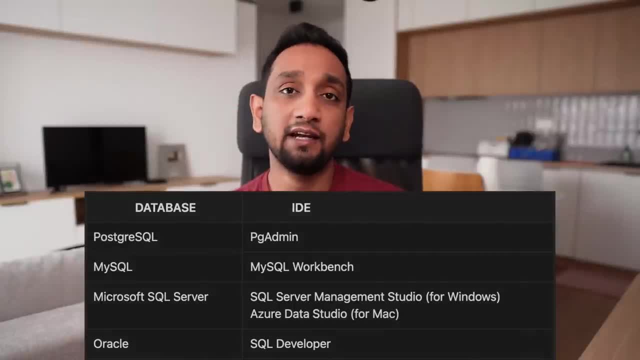 using Mac, then it comes with Azure Data Studio And when it comes to MySQL, you have a tool called MySQL Workbench which you can install in order to work with MySQL. And when it comes to PostgreSQL, you have a tool called as pgAdmin which basically you can use to connect to your PostgreSQL and start. 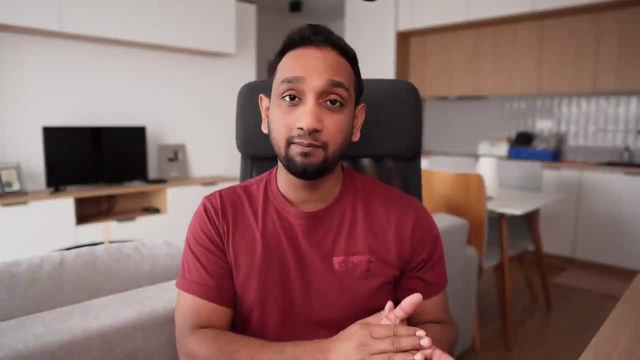 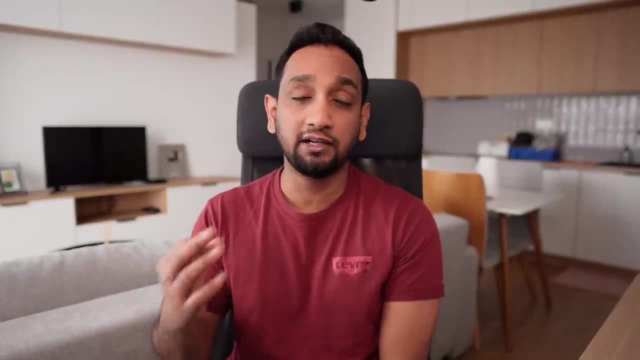 working. Okay, So this is a prerequisite. So let's say you have a database and you want to have a database installed and have an IDE installed. If you're using a cloud-based database or data warehouse, then make sure that you have set up them in your browser, right? So 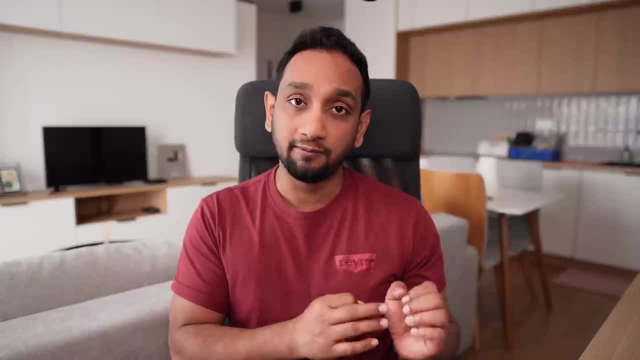 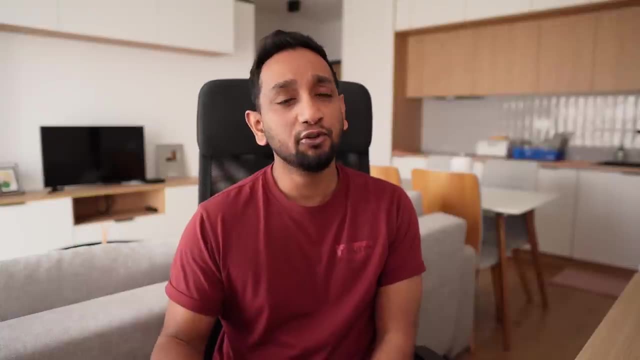 once all of this is done. basically, this is the only prerequisite that you need. If you're watching this video, then you probably are interested in getting into data analytics, data science, software engineering, and you know that SQL is a very important skill. but SQL is not. 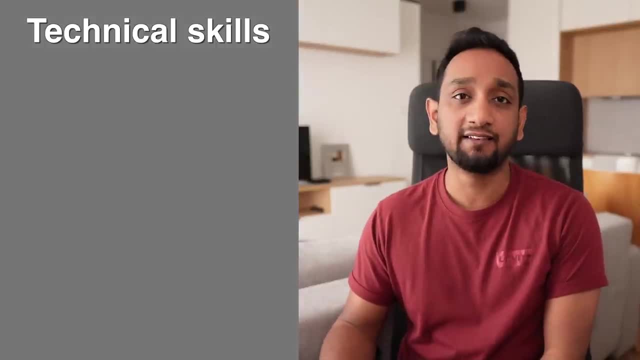 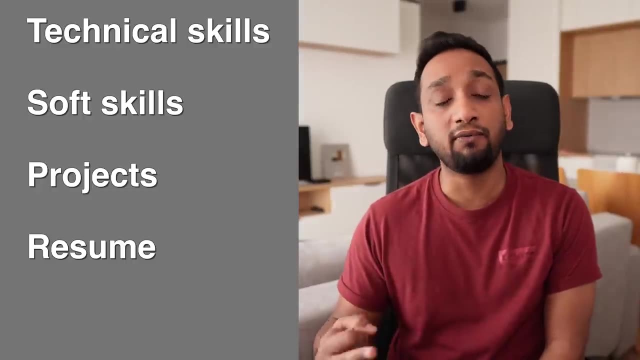 the only skill right. There will be a few other technical skills that you will need to learn. You also need to have certain soft skills. You need to build portfolio projects. You need to have a good resume. You need to know how to effectively search for a job right Now- an easier way of. 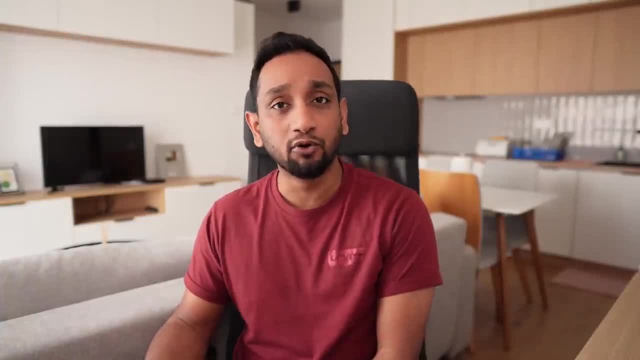 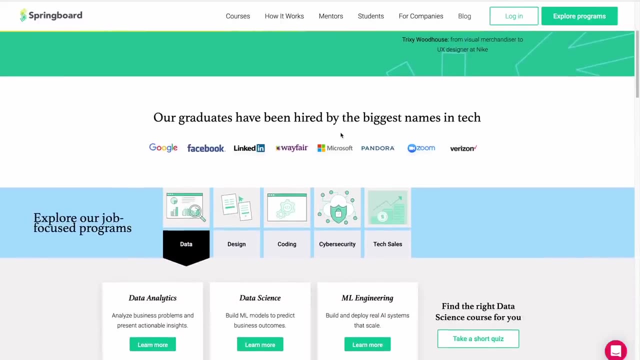 doing all of this in one place is by doing a bootcamp course on Springboard. Now, Springboard is an online platform that offers bootcamp courses related to data analytics, data science, software engineering, UI, UX design, et cetera. Now, just to give you a quick overview of what 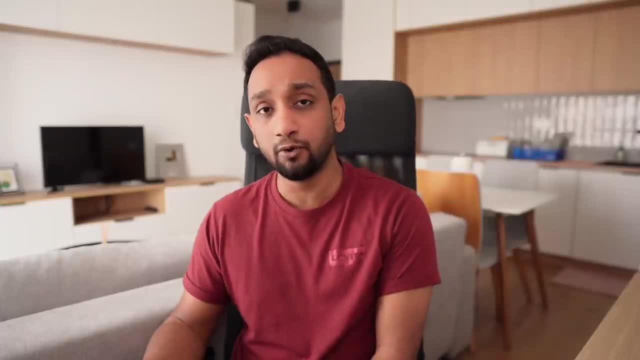 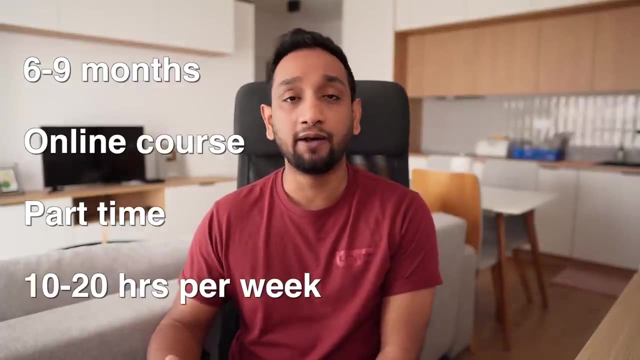 exactly happens in a data analytics bootcamp on Springboard. Now the course Springboard. it spans for around six to nine months. You can do it online, part-time, by spending maybe 10 to 20 hours per week During the span of this course, you would, of course, be learning all the technical. 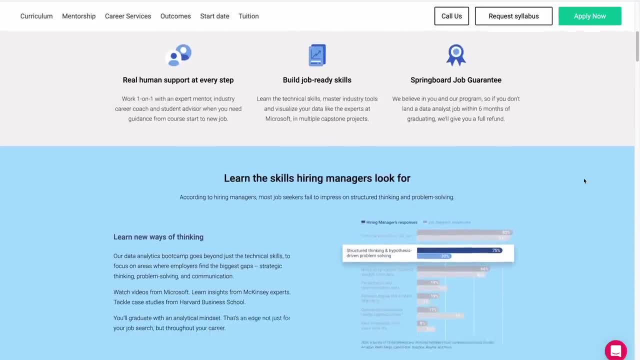 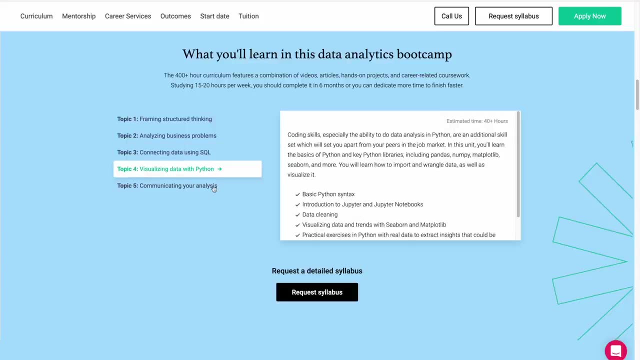 skills that is required to get into data analytics, like Python, SQL, data visualization tools, et cetera. You would also be learning some very important soft skills like improving your communication skills, business analysis skills, problem solving skills and, more than anything. 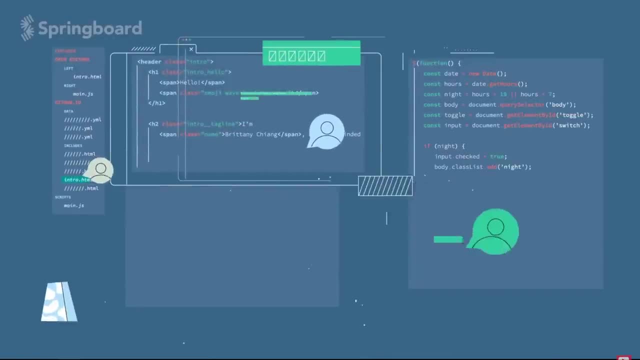 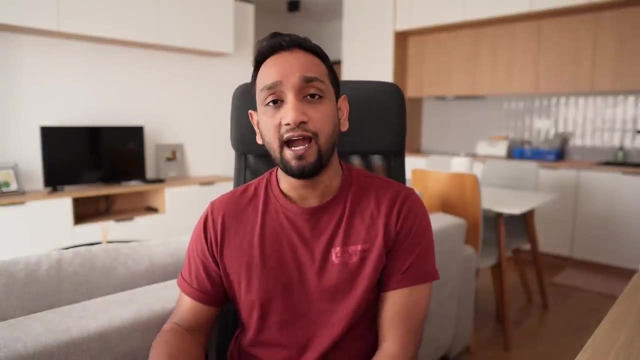 you would kind of get that analytic mindset which most of the employers are currently looking for. Now, once you have gained all of these skills, you would then be assisted in building portfolio projects, And, when it comes to projects, you would be given the option to choose your own data set. 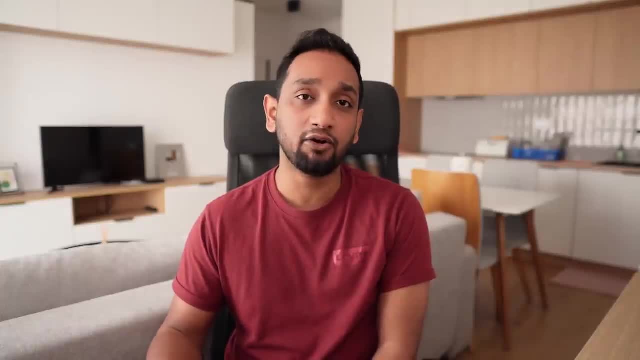 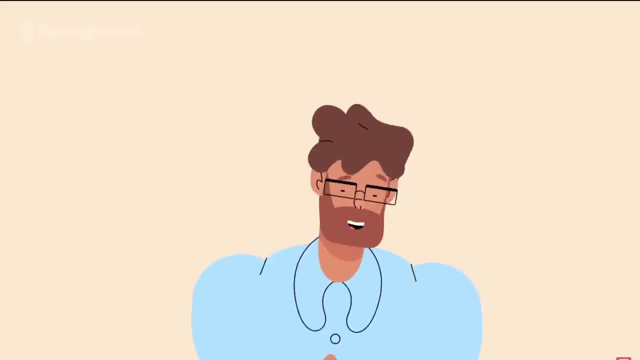 based on your interest. Once the projects are ready, you would then be assisted in building your resume, and Springboard will also assist you in your job search. Now, if you qualify for the job guarantee program offered by Springboard and you're unable to find a job in the set period, 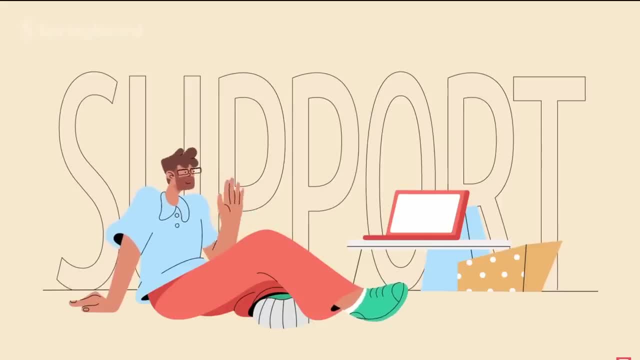 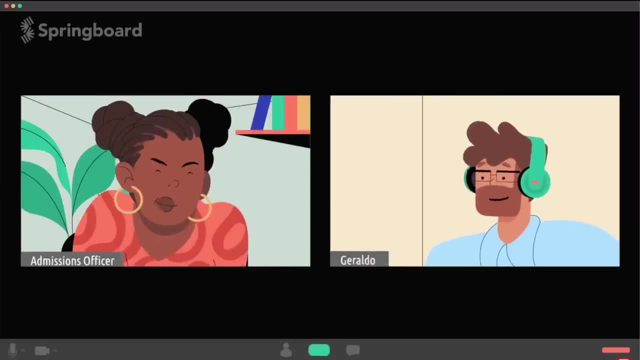 then Springboard will give you a full refund. Now, in addition to all of this, Springboard also offers a one-to-one mentorship program, where an expert will be allocated to you So you can have a one-to-one discussion with them, ask for any questions or clarify any doubts or ask for any. 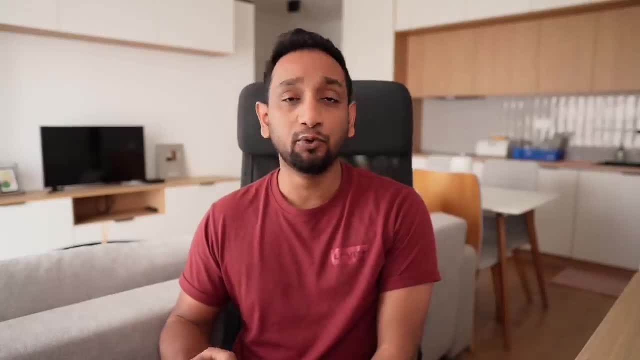 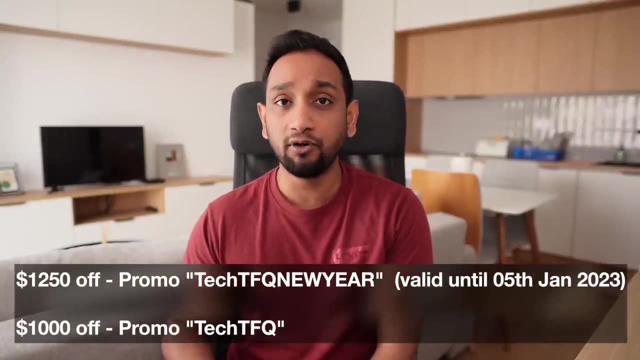 assistance with your mentor. So if you are looking for a bootcamp course, then I would highly recommend you to check out Springboard. All the details are present in the video description. You would also find a couple of promo code. There is a promo code that will last until. 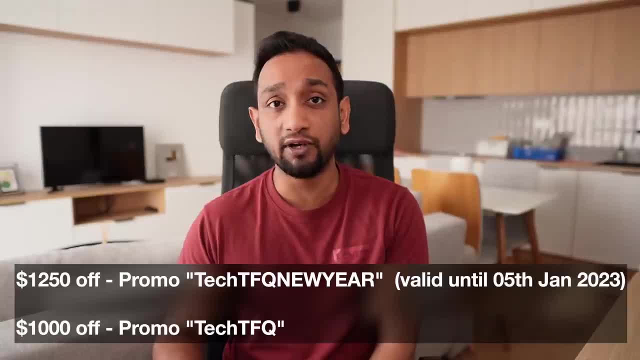 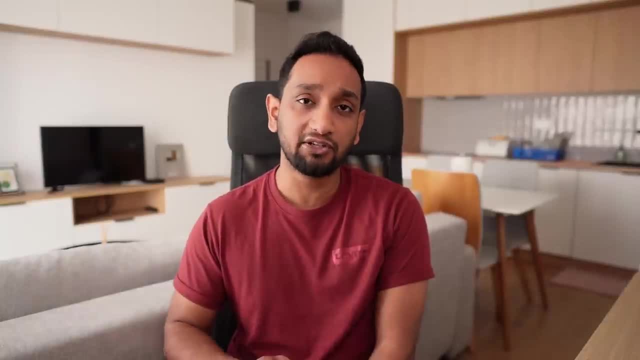 the new year, which will give you a $1,250 off on any of the courses, And there's another promo code for any courses that you take on Springboard. So definitely check out the video description for all the details. So you have understood the prerequisites. Now let's look at how you can. 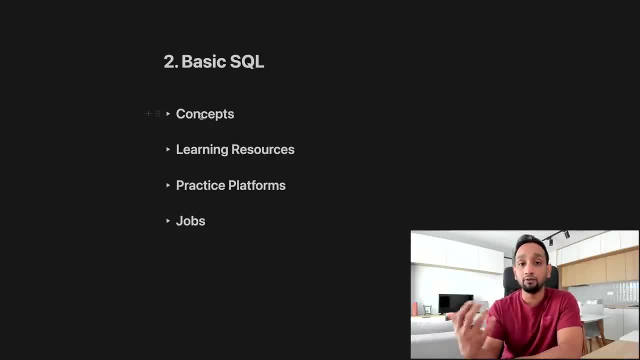 learn basic SQL. First, I'm going to cover all the concepts you will need to learn. We'll then see the free learning resources and the platforms where you can practice. Finally, I'll talk about the jobs that you can target with basic SQL skills. Okay, So the concepts that you will basically need. 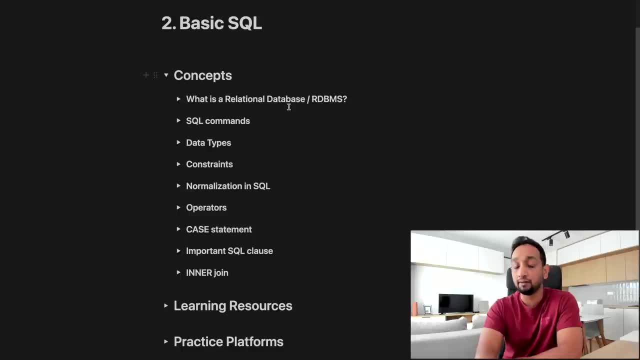 are. first of all, you kind of need to understand what is a relational database and what RDBMS are. Okay, Okay, Okay, Okay, In a relational database, what is a schema with respect to relational database? right, Once you have this basic understanding, then you can look at all the different SQL commands. 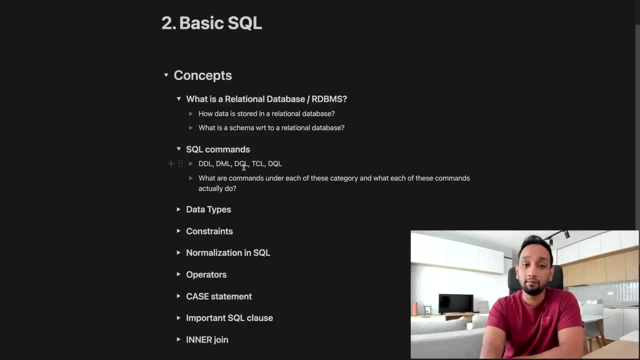 Now they basically there are five different categories: DDL, DML, DCL, TCL and DQL. Now, under each of these categories there are several different SQL commands. Each of these commands are meant to do certain specific tasks, So you need to kind of understand what each of these. 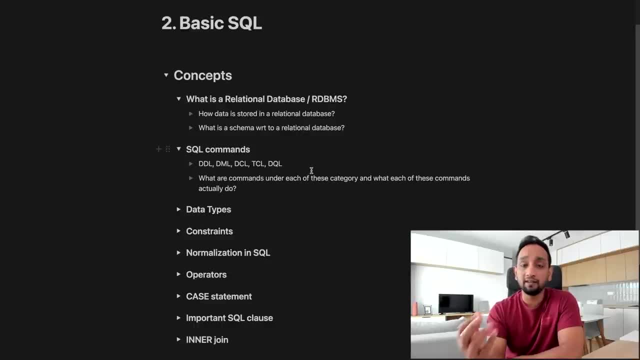 commands will do Okay, And it's also important to understand the difference between certain commands, like drop, delete and truncate, because some of you guys might get confused that they look similar but there is a difference between each of these commands, So it's better to understand all of these commands clearly, Okay, So once you are thorough with SQL, 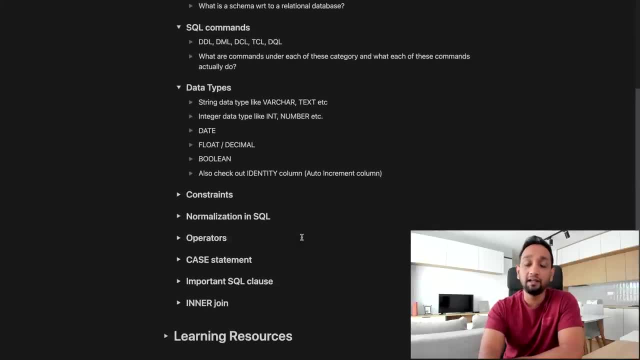 commands, then it's time to understand what are data types, right? So when it comes to data types, there are like hundreds of different data types. You don't need to learn each and every data type. Primarily, I would say these five type of data types. So string data types, maybe varchar. 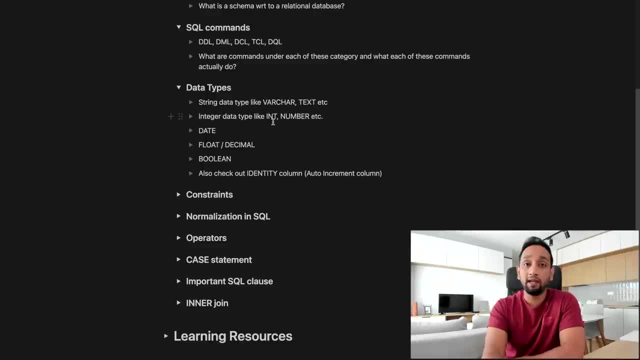 text or something else. Okay, So string data types, maybe varchar text or something else. And then integer data type, maybe int number or something else, maybe specific to your database. right, Then you need a date data type. You need to understand how date is stored in a table using 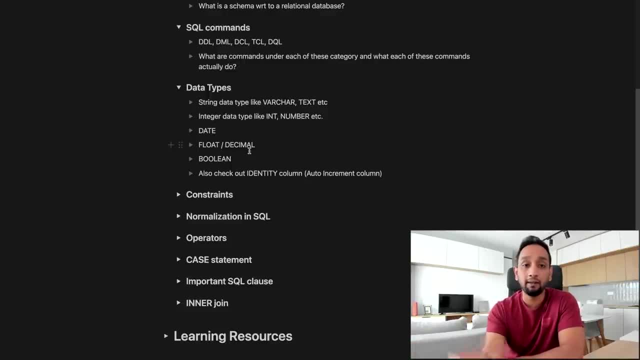 this date data type, Then float or decimal data type, Then finally Boolean data type. Now, Boolean is not supported in every RDBMS, So you might have to check that out. And additionally, I'd also ask you to understand what an identity column is Now. basically, if you want to auto, 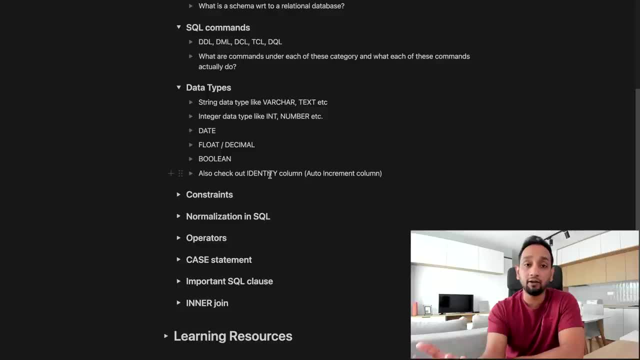 increment a column, you can basically define the column as an identity column. So it's good to understand how you can define a column as identity column and how you can basically load data into that or modify data into a table which contains an identity column. Okay, So once. 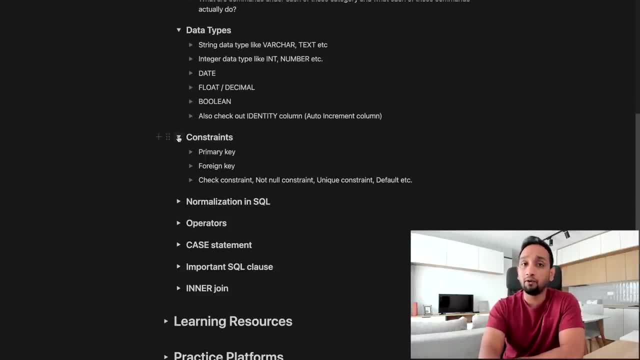 you have this basic understanding, we'll then look at a very important concept called as constraints. Okay, Now, in constraints, there are several different types of constraints, but primarily you need to understand what is a primary constraint and what is a foreign key constraint. 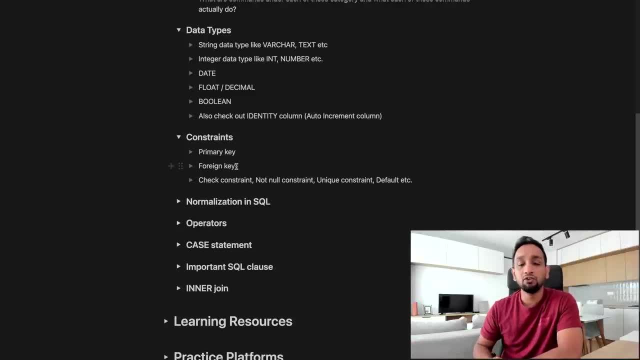 Okay, These two are very, very important. Without understanding this, you should probably not proceed To learning anything else. Okay, Now, in addition to this, there are check constraint, not null constraint, unique constraint, default constraint. It's good to understand these as well. 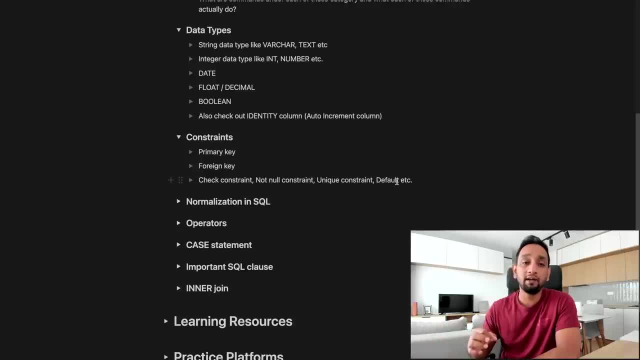 Okay, Of course there will be other constraints as well, but I would recommend to first understand all of this and not worry about each and every constraint that is available. So once you are thorough with constraints, then you can understand normalization in SQL. 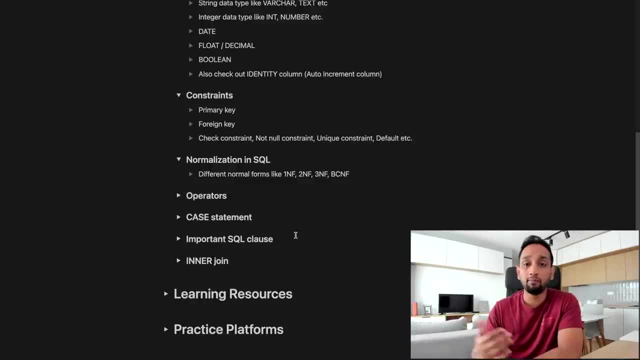 Now there are different normal forms: first normal form, second normal form, et cetera. It's good to understand. why do you need to make your database normalized, Like how does it help and what are the different rules present in each of these normal? 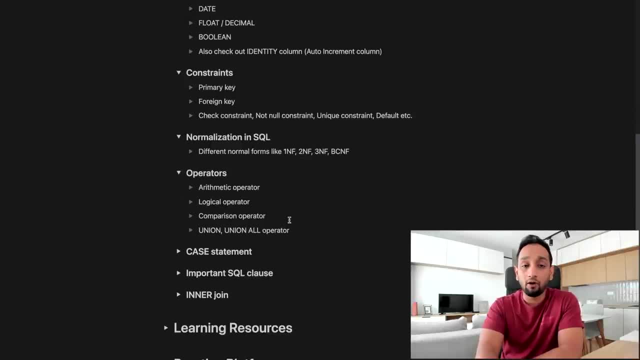 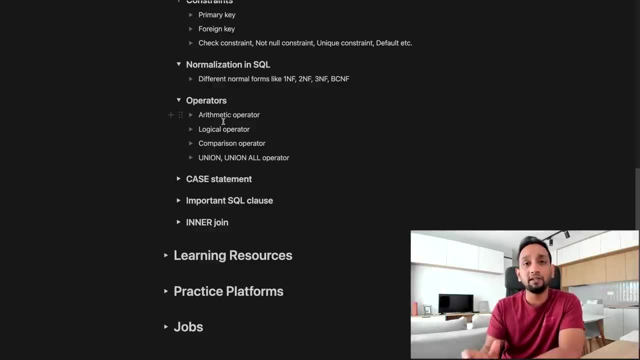 forms. Okay Now, after that, you can look at operators. Now there are several different types of operators. You don't need to learn each and every operator, but these most common operators are something that you would basically use in each and every SQL query that you write. 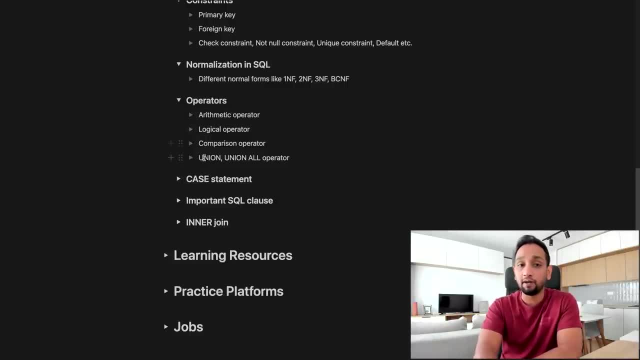 So arithmetic operators, logical operators, comparison operators, union, union, all operators, Okay, So just focus on these operators to start with. And then, of course, you need to know what is case statement, not just simple case statement, but how to write nested case statement, That is, a case statement inside another case statement. 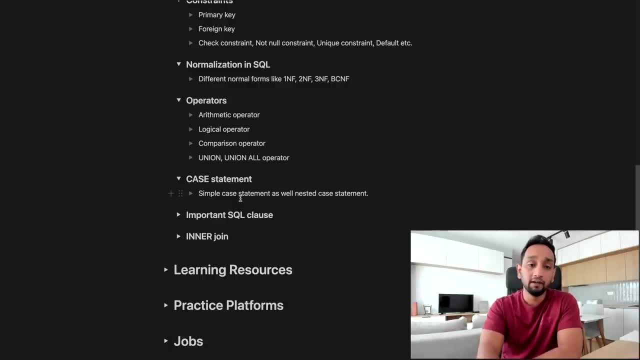 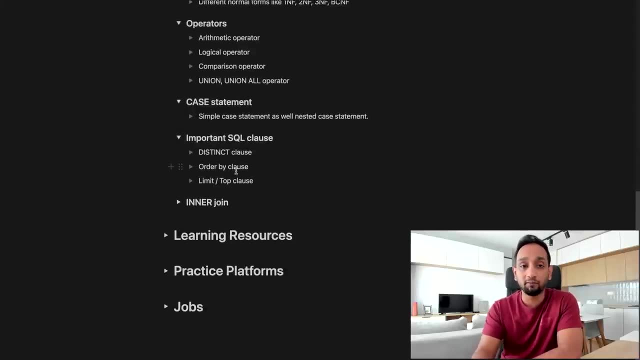 right. Just try to understand that. it's very simple. And once you are thorough with that, then there are certain important SQL clauses like distinct clause, order by clause, limit or top clause. Okay Now, limit is basically used in most of the RDBMS, but I think in Microsoft. 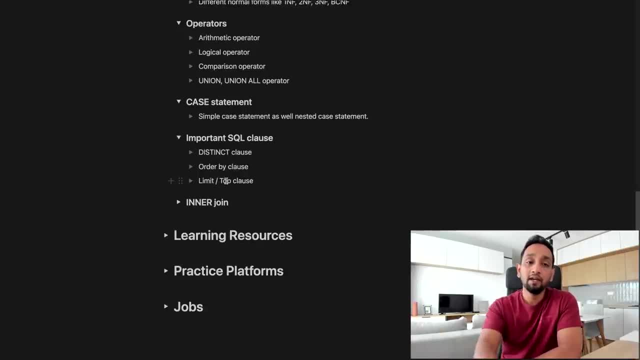 SQL server. instead of limit, you will need to use top. Okay, So basically, just try to understand what each of these clauses are meant to do, And I think that should be pretty good. And then, finally, inner join. basically, If you want to fetch data from multiple tables, how do you do an inner join, right? So these are. 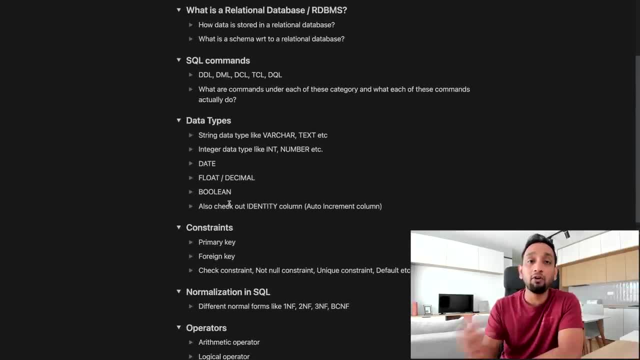 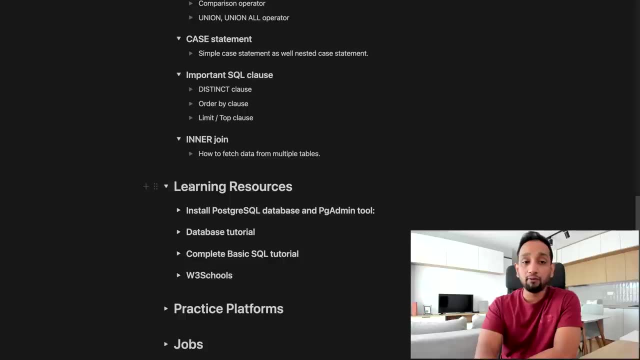 all the different concepts that you will need to learn in order to call yourself that you have basic knowledge of SQL. So these are the concepts that you will need to learn for basic SQL, And the resources that I would recommend is, first of all, you need to install a database And if you want to, 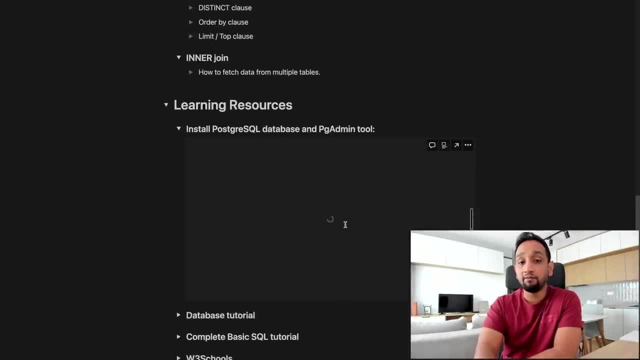 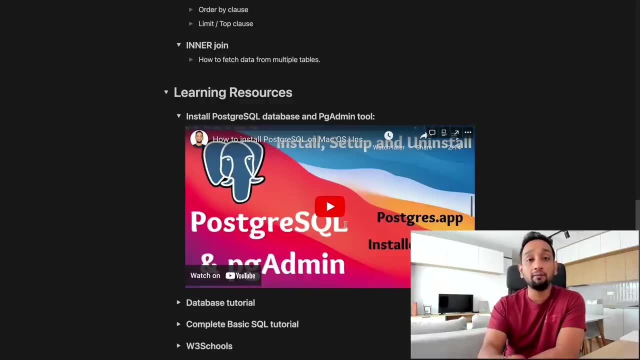 install PostgreSQL or PG admin tool, then I have created a video on this channel itself, which I think is pretty clear. You can just follow these steps to install PostgreSQL. I have done this in the past, but the same process can be followed in windows as well. Okay, And once you have installed, 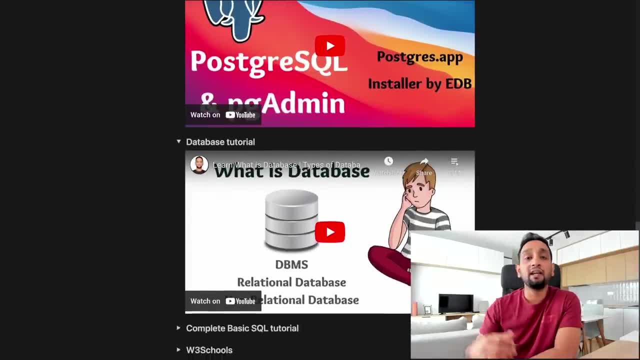 your database and your ID is set up, then the next thing is just to understand what exactly a database is. Now, SQL is used in relational database, but there are non-relational databases as well. It's always good to understand what a database is, what data is, how data is stored. 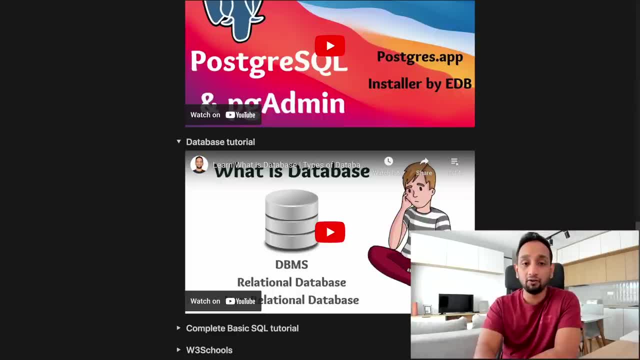 all these basic things, but it's going to be very useful for you in feature to understand these concepts. So I have created this video about databases. I would highly recommend you to check out this video. And then, finally, we have the database. So you can see that we have a database. 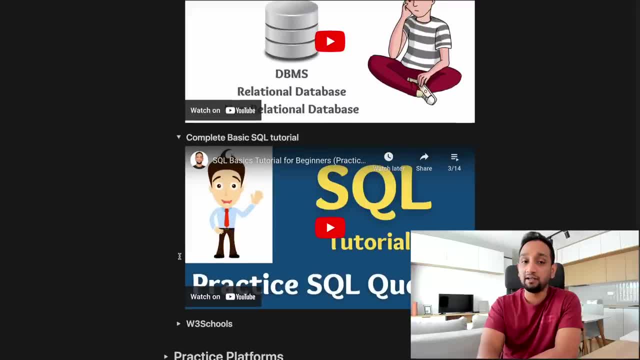 once you have installed your database, once you have understanding of all this relational database, then it's time to basically watch this SQL basics tutorial video. I have created this video, which covers all of this basic SQL functionalities or concept that I just mentioned. 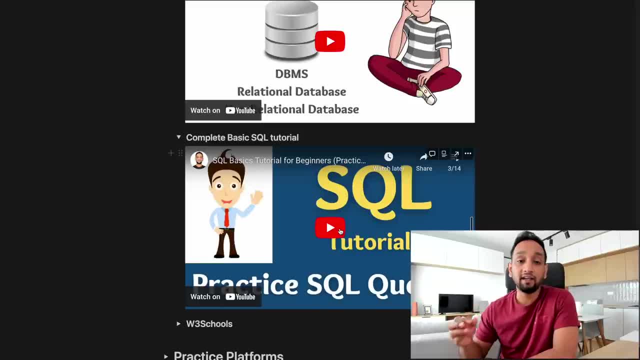 Okay, So in this video you will also see that I'm using a data set, and I have basically placed the script of this data set in my blog. You'll find a link to that sample data set in my video, So you can then use that data set to make your own practice right. 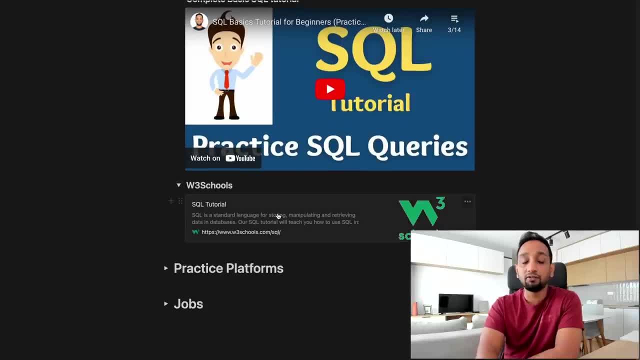 Now, other than this, another resource that I would highly recommend is W3 schools. I'm sure most of you guys would have heard about this. Now, this is a fantastic platform. You can basically find the syntax to all of the different concepts that I just mentioned here. Okay, So I would. 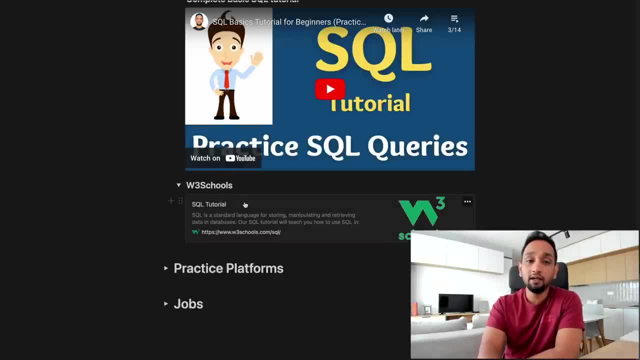 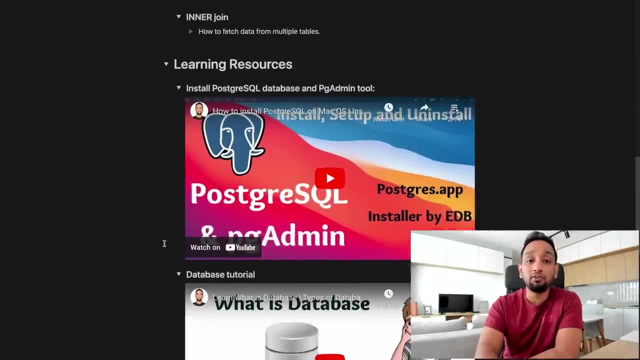 I also recommend you to check out this particular platform. Okay, Now, once you have learned all of this basic concepts, the next thing is you will need to practice writing SQL queries, where you will be using all of these basic concepts right Now. in order to practice, I would recommend these: 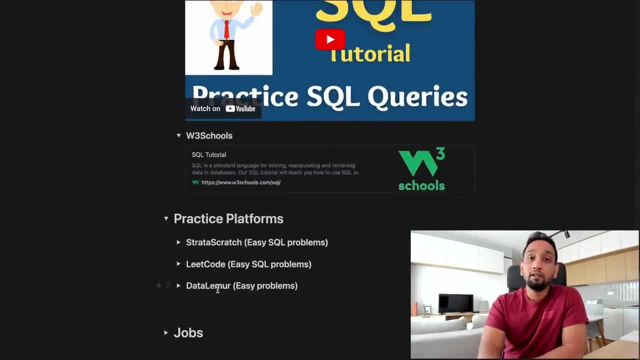 three platforms: Stata, Scratch, Leadcode and Data Lemur. Now, in each of these platforms, you will find easy, medium and hard problems. Now, since you are only looking at basic concepts here, I would only ask you to solve problems which are of easy difficulty level. So go to Stata Scratch. 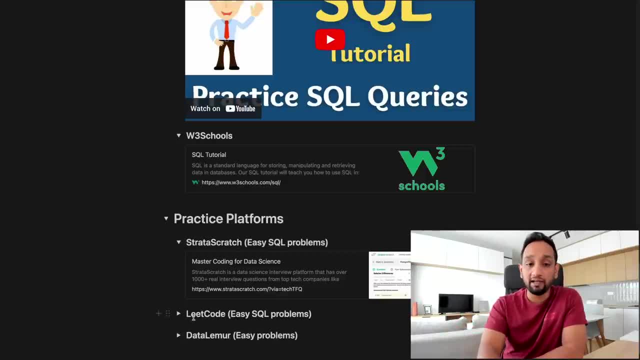 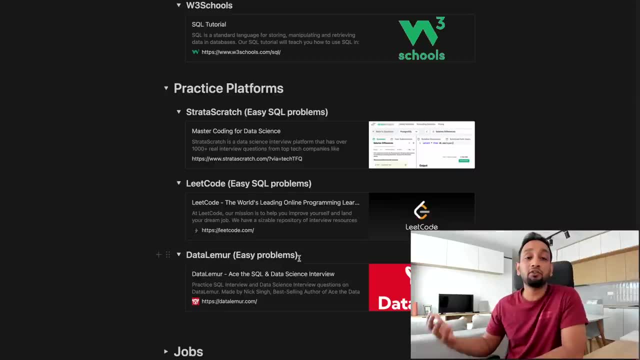 and just search for easy problems on SQL and you should be finding it. And same way you will find easy problems on Leadcode, and the same thing in Data Lemur as well. Okay, So these are the three platforms where you can solve SQL queries. Choose the easy ones and probably you will be able to. 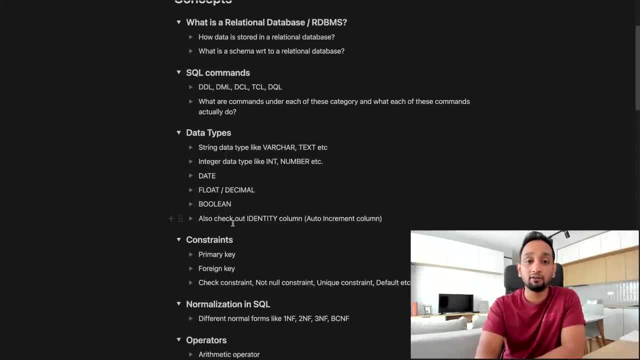 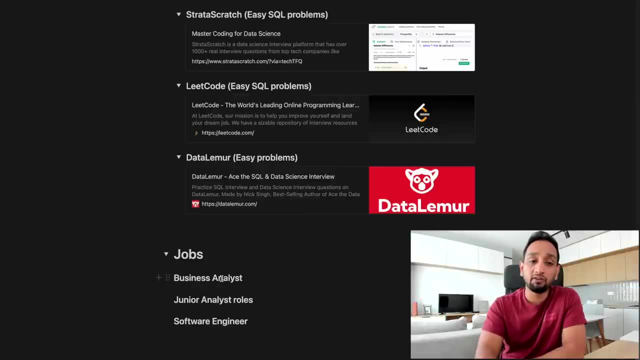 solve most of those problems if you are comfortable in these concepts. Now let's see what are the jobs you can target with basic SQL knowledge. Now, basically, I would say if you are looking for a business analyst role or a junior analyst role- when I say junior analyst, it might be any type- of because there are so many different types of analyst right. So any junior analyst role, I think the SQL, the basic SQL, should be more than enough. And then also software engineers, maybe not senior software engineers, but a normal, I think, up to 1,, 2,, 3 years of software engineers. 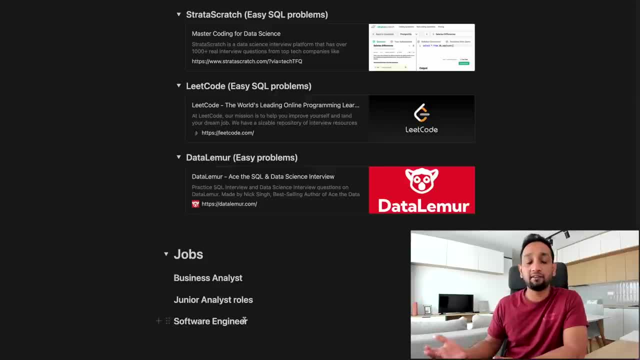 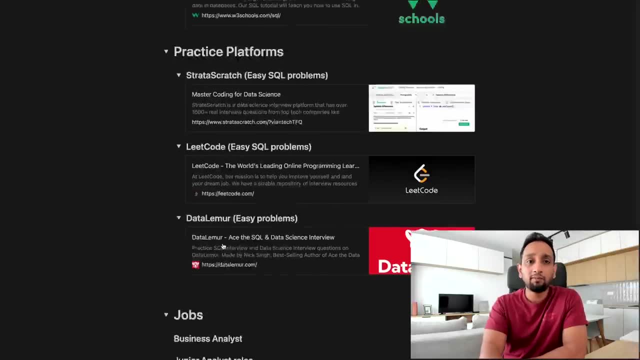 to use or write sql queries or insert scripts or update scripts in order to connect to the database, and i think basic knowledge of sql should be enough for them. okay, so this is basically how you can learn basic sql: all the different resources and the platforms for practice. okay. 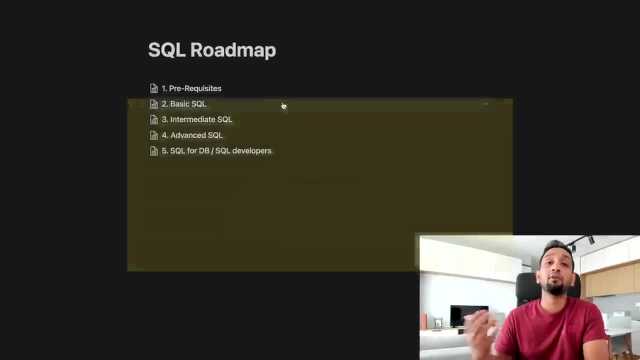 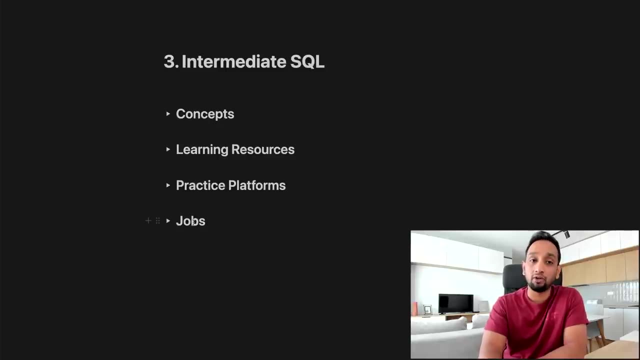 now let's go back and look at what you need to do if you want to learn intermediate level of sql. okay, now again i'm going to cover the concepts and then we'll look at the resources, platforms and jobs. okay, maybe in this case, first let's look at jobs. so, basically, who should be learning? 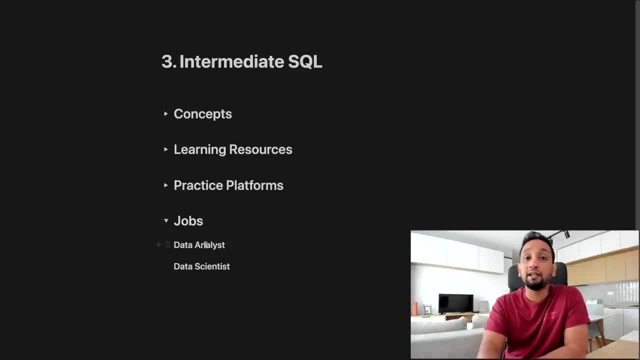 intermediate sql right, especially if you're looking for a data analyst role or a data scientist role, then i think just basic sql will not be enough. you would have to learn the intermediate level of sql as well. okay, so when it comes to intermediate level of sql, mainly you will 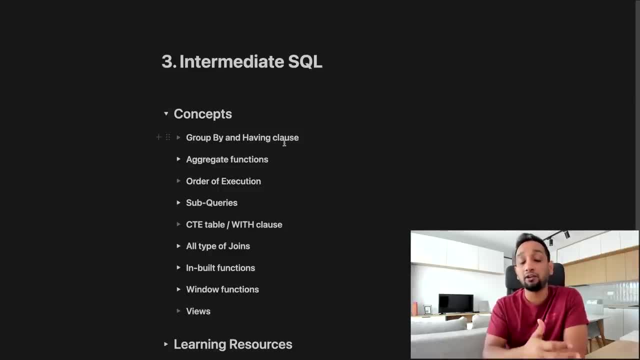 need to learn group by and having clause. i know many of you would argue that group by and having clause should have been part of the basic sql, but the thing is there are several complex questions related to group by and having clause. but the thing is, there are several complex questions. 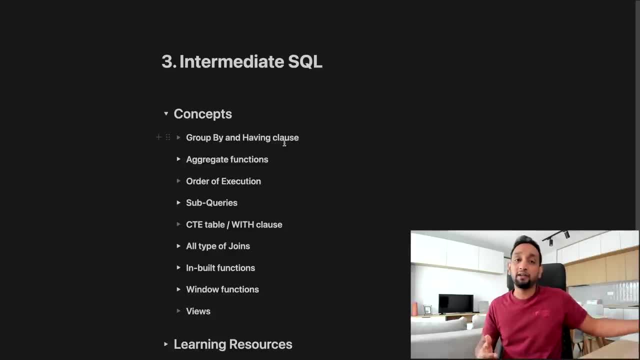 that you can write using group by and having clause, and that is why i didn't want to put that as part of basic, but as part of intermediate. you definitely need to know group by and having clause. you also need to know how to use aggregate functions- min, max, average, sum and count. okay, and 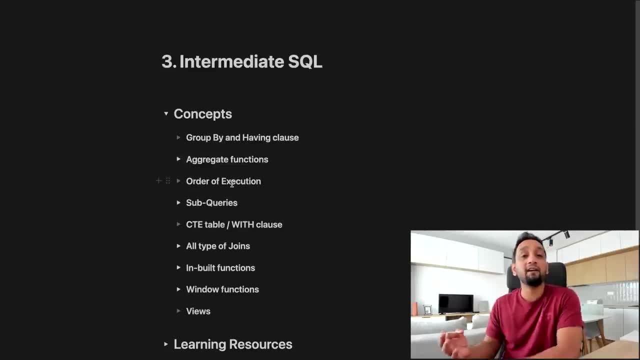 then you also need to know order of execution. it's not like mandatory, but by knowing order of execution you it will be very helpful for you when you are trying to understand a already written query or sometimes when you're stuck. order of execution is something that can help you to. 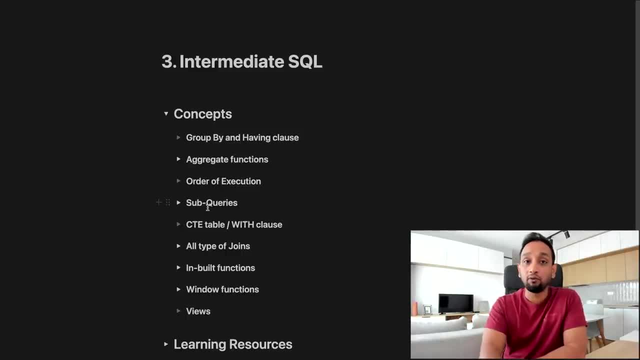 get unstuck okay. so so definitely, you will need to know sub queries. it's a very, very important concept. you will need to know ct table or with cross. you, of course, need to know all the different type of joints, all the outer joints- left join, right join, full outer join. you will need to know cross join. 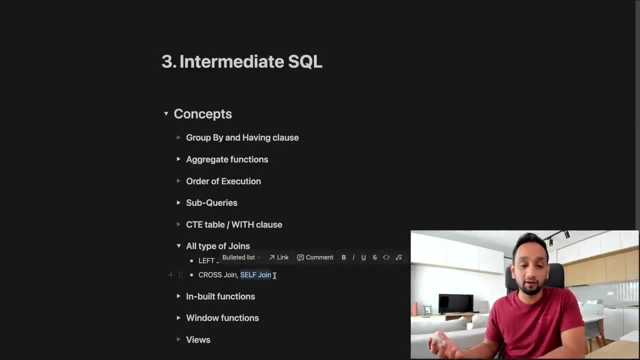 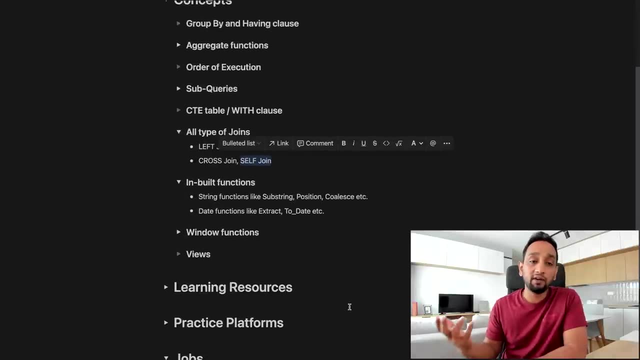 and, more importantly, you need to understand how a self join works right. self join is very important. you should definitely be comfortable with that. and also you need to learn certain inbuilt functions. now, mainly, you can learn certain string functions as well as date functions- mainly functions where 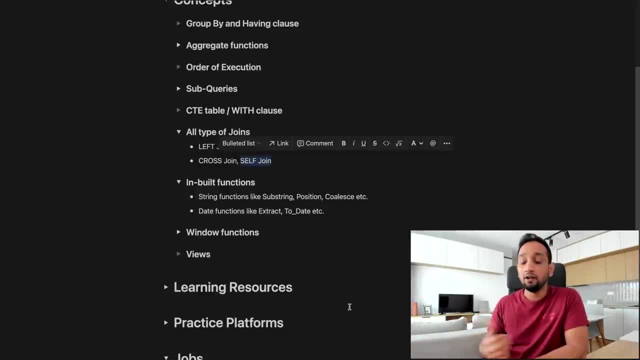 you will need to extract a month from a date, or you need to reformat a date, or you need to fetch a substring from a string, or replace a null value with some other value. so these are the different types of inbuilt functions are present in every rdbms, so, based on whatever rdbms you are learning, 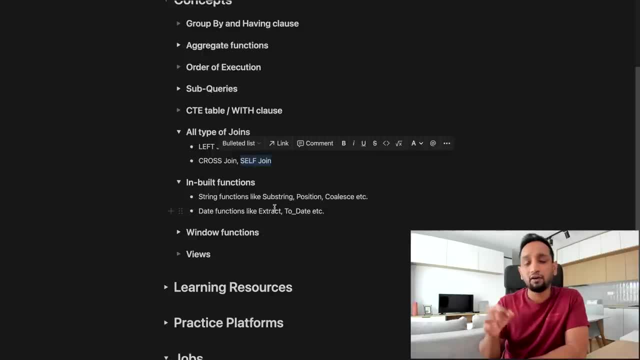 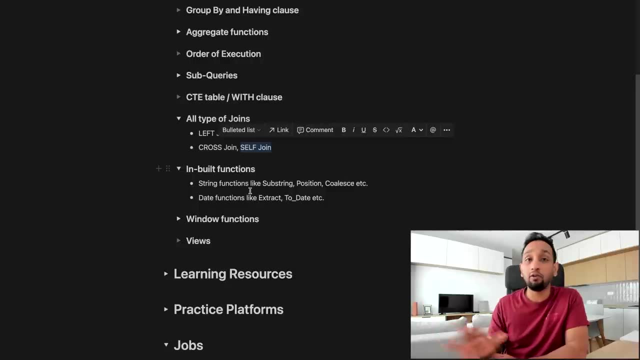 you will need to get hands-on with, or remember, very important inbuilt functions. okay, now i'm going to provide you a resource where it's a very good resource, where you will find a list of all the inbuilt functions. uh, a lit in a short while, okay, and then finally, 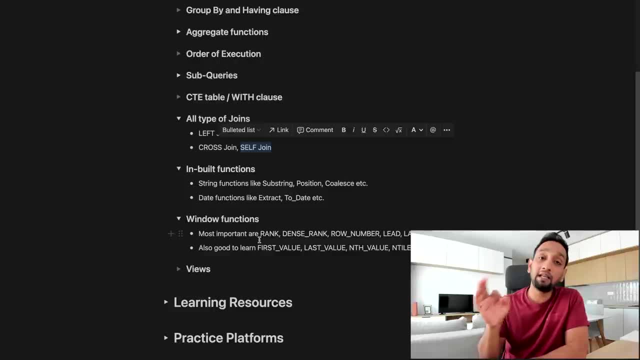 a very important concept is window function. you should definitely learn window function without knowing window function. i don't think so. you will basically be able to survive as a data analyst or a data scientist. okay, now in window function. there are a lot of window functions, but the 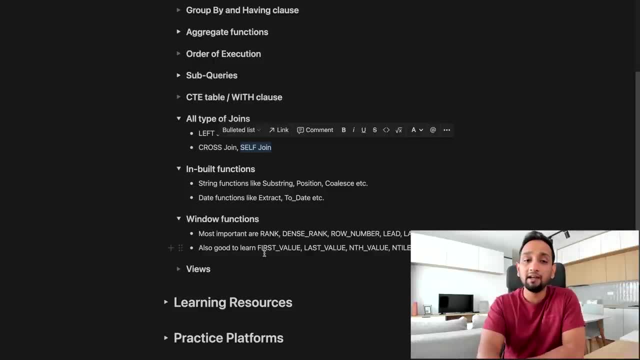 most important would be rank, dense, rank, row, number, lead, lag, but also first value, last value, nth value, entire, are also very much used. okay, now, finally, you also need to understand what are views and why are they used. okay, so these are all the different concepts that you will need. 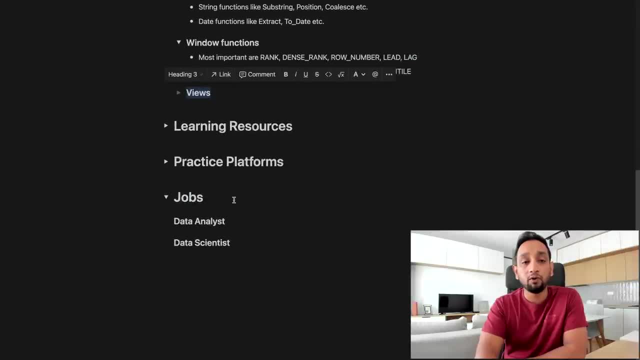 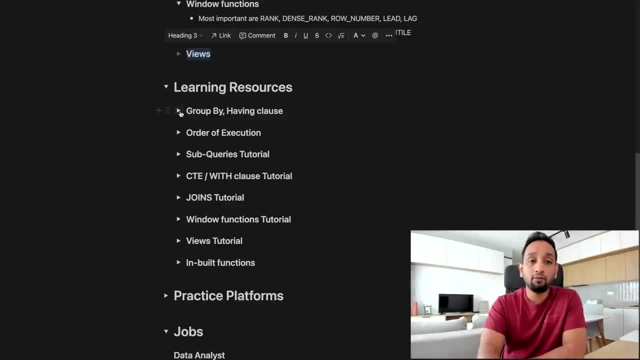 to learn in order to get intermediate level in sql. now, if you ask me what are the resources for learning all of these concepts? i basically have created tutorial videos on most of these concepts. so for group by and having clause, i have not created a video, but i would recommend you to. 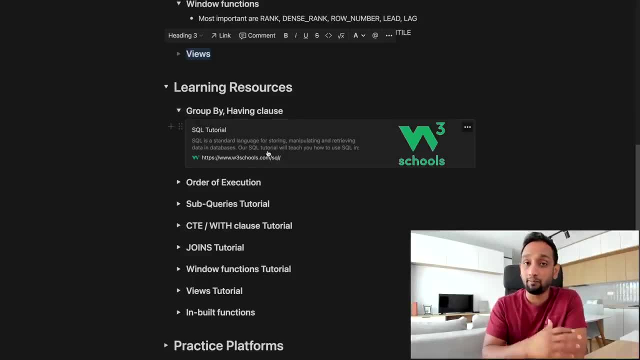 check out w3 schools. it's a fantastic platform. as i mentioned earlier, you have pretty good examples for group by and having clause. i think this should be more than enough for you to understand the concept. but let's say you want me to make a tutorial video on group by and having clause. 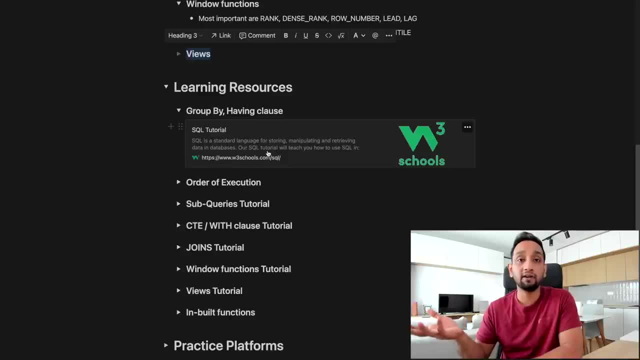 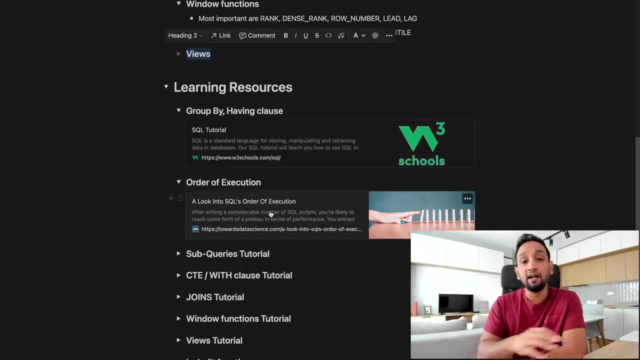 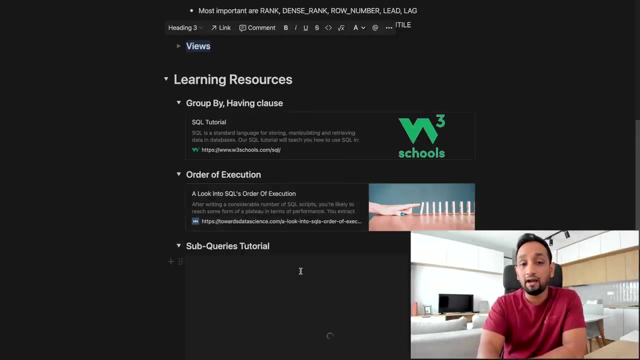 then definitely mention that in the comments below. maybe i can cover a tutorial video on this concept as well. for order of execution, there is a blog that i found very interesting. i'll leave the link to this blog. in fact, i leave the link to all of these resources in the video description or in my blog. okay, so for sub queries i have created. 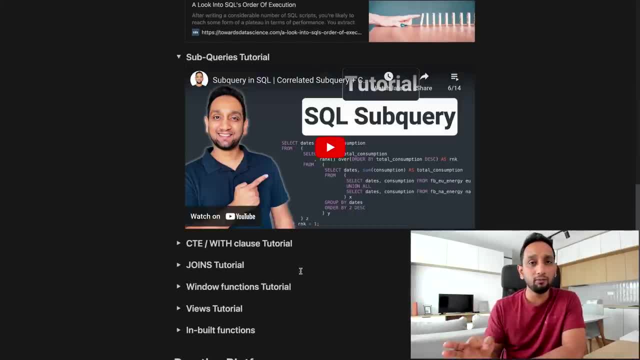 a fantastic tutorial on youtube. this is one of my most successful videos on this channel. i know it is very good and all the concepts are very well explained, so i would highly recommend you to check out this tutorial video. with regards to with clause or city table, again i have created 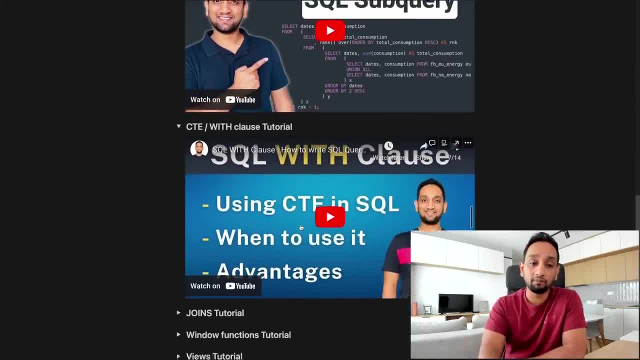 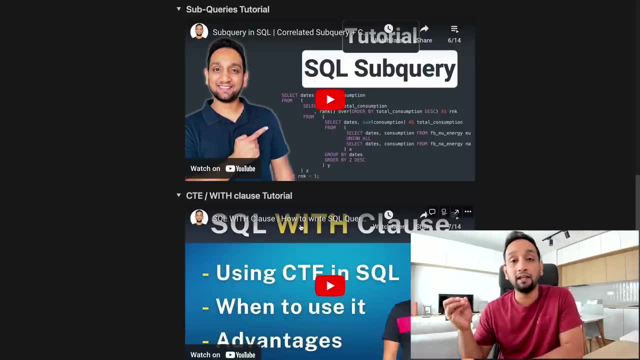 tutorial video on youtube. i would recommend you to check this video. okay, and and the best part is, whatever scripts and data sets i'll be using to explain this tutorial, i will leave a link to that script in my blog so you can download that script and practice it yourself. okay, just 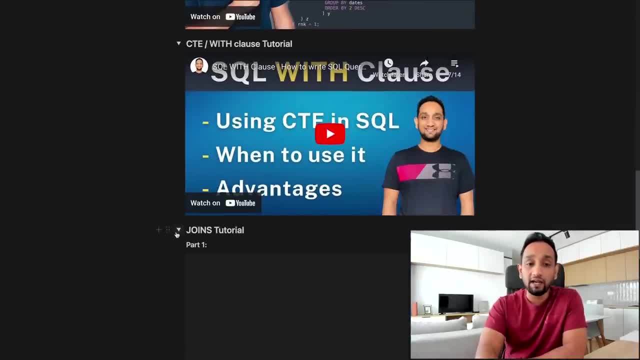 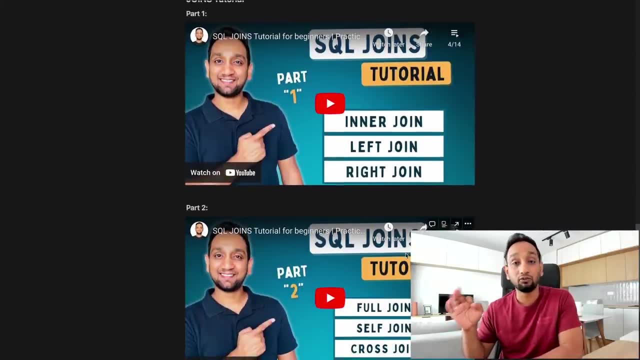 check the video description for all the details. when it comes to joints, i had created two videos, part one and part two, where i have covered all type of joints. these are one of the best videos or resources you can find to learn joints. i can guarantee you that. so definitely check out these. 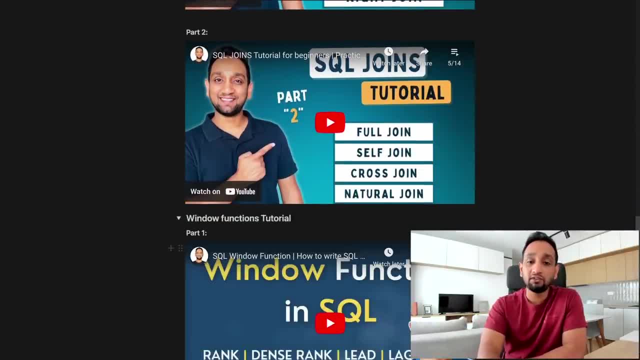 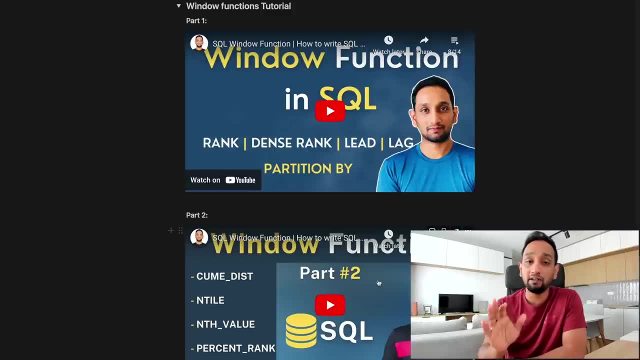 two videos to learn about joints. when it comes to window functions, again i have created two tutorial videos, part one and part two. again i have covered all the different window functions that are available in sql in these two videos. they are very good. these are very successful videos. 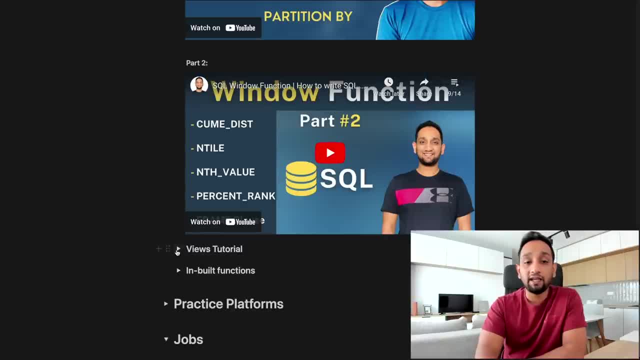 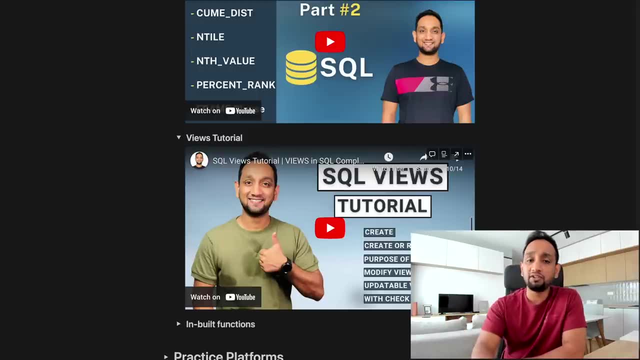 i would highly recommend you to check that, check them out. when it comes to views, again, i have created a views tutorial video where, basically, i have covered concepts which you might have never used in views. so definitely check out this tutorial video on views in my channel itself. 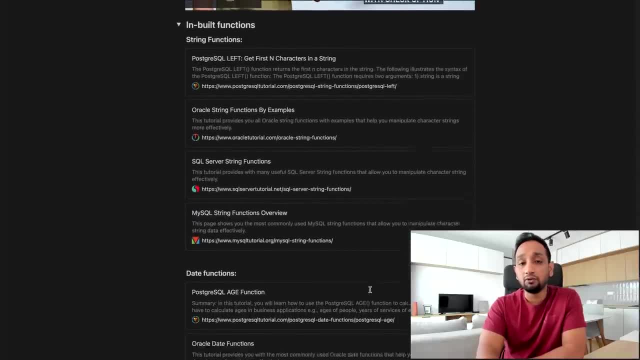 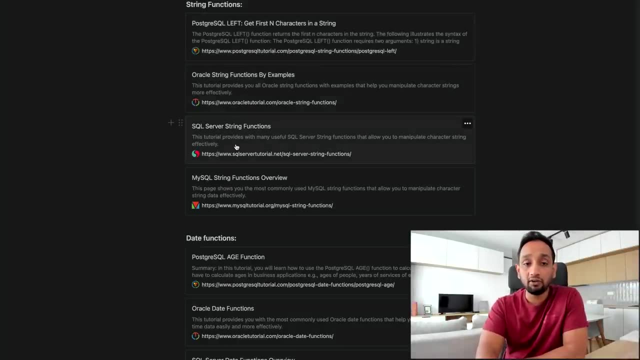 and finally, when it comes to inbuilt functions, i'm going to leave a link to a couple of blogs where, basically, you will find all the different inbuilt functions available in oracle: uh, possibly sql, sql server and mysql. okay, so both string and a date function. so i 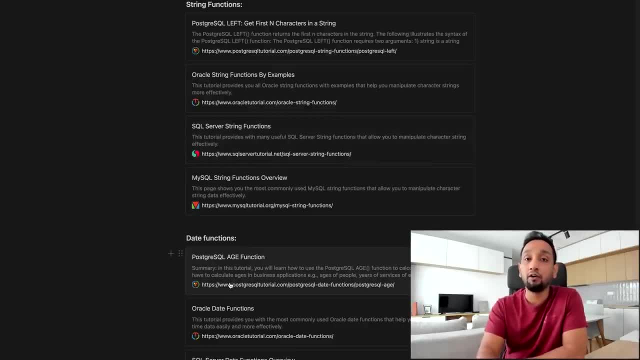 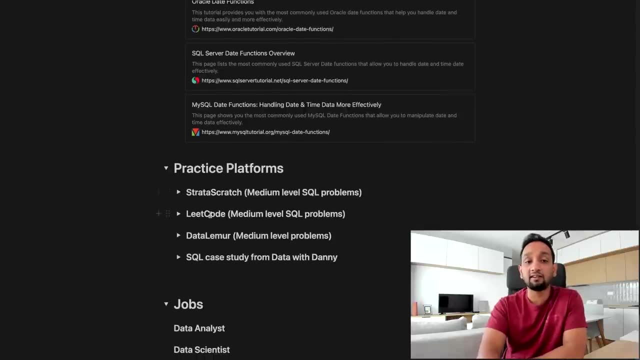 would definitely recommend you to go into this blog in order to understand all the inbuilt functions. okay, and for practicing these concepts, i would recommend four platforms again: status, scratch, leadcode and data lemur. in this case, try to solve median level sql problems. okay, and after that, one additional resource i would recommend is: 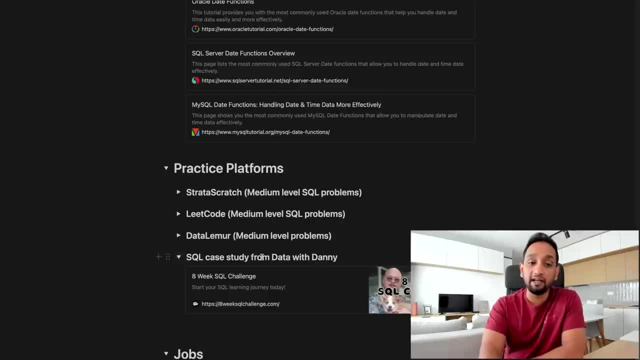 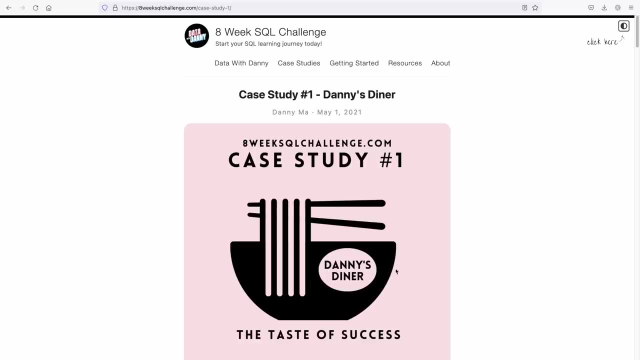 the sql case study from danny data with danny. uh, it's a fantastic platform here. if you go, you would basically find, i think, eight case studies and if i just open the first one, you would basically see that case study is something like: you have a scenario you need. 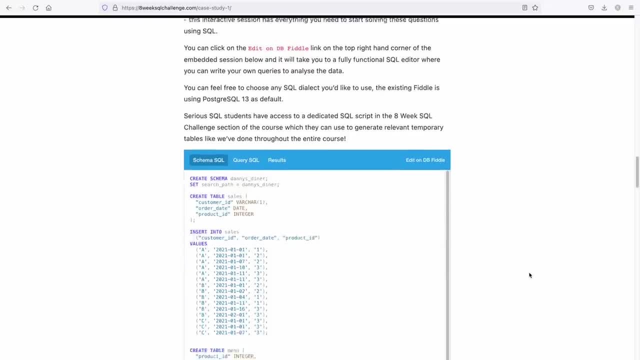 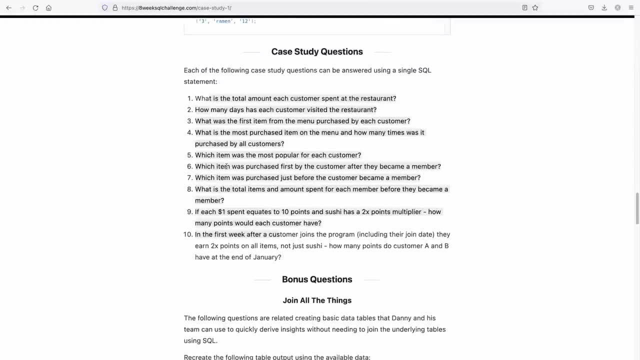 to understand the scenario. you have sample tables and data given and then, based on that scenario, there are certain problems you will need to solve by writing sql queries. okay, so these case studies are very useful. you will kind of get an end-to-end picture of how you should be going about. 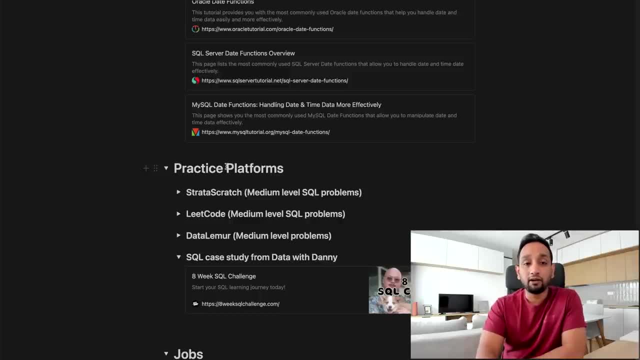 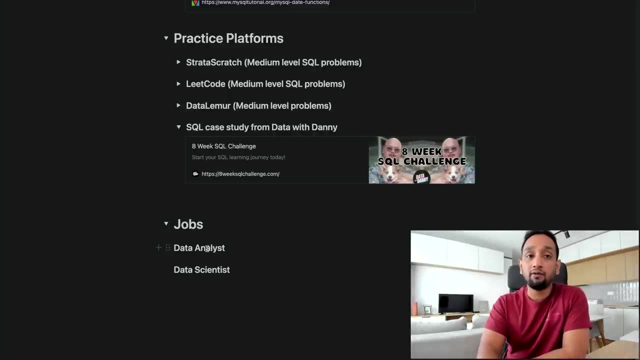 a problem and then solving a problem. i think these are the platforms that i would recommend for intermediate level of sql and jobs i already mentioned. if you're looking for data analysts or data scientists, then this is the intermediate level of sql- is what you should be learning. 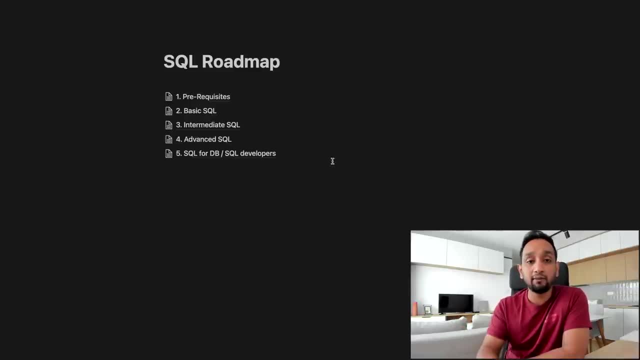 now let's look at what you should be doing if you already have basic and intermediate level of sql knowledge and now you want to basically get advanced level of sql knowledge. right. in this case, the jobs that you can target by learning advanced sql is basically like a data engineer. 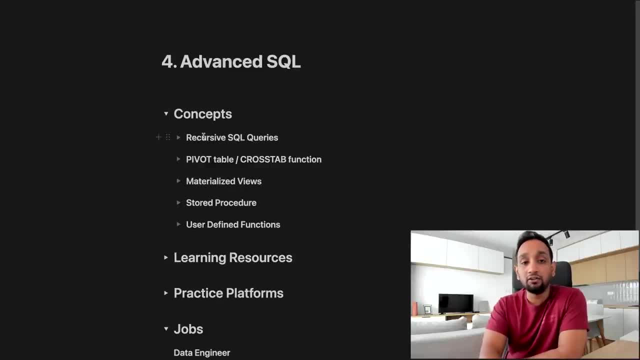 right and the concepts that you would additionally need to learn are you need to understand recursive sql queries. you need to understand pivot table or crosstab. now, pivot is something that is supported in mysql. i think not supported in mysql, but supported in microsoft sql server and in oracle. 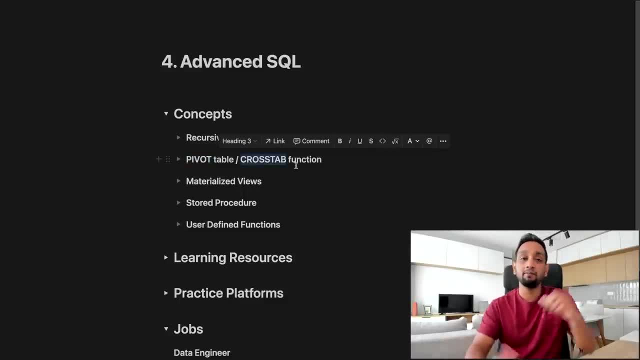 and crosstab is supported in postgresql kind of does the same thing, but in postgresql you will need to use crosstab, and in mysql, both of these are not supported. you can perform the same thing using case. okay, and i'm going to mention a resource where you will basically learn all of that. okay, in. 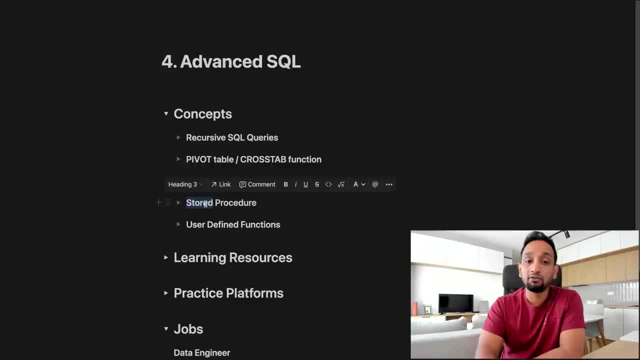 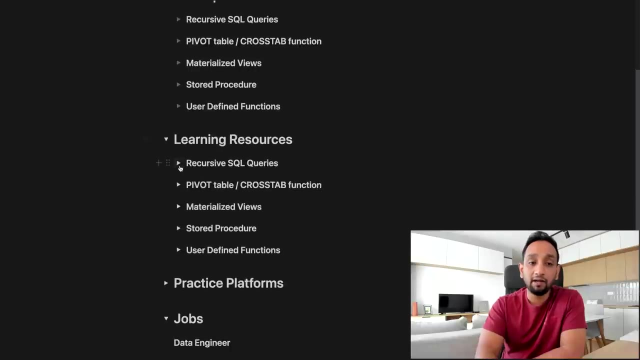 and you also need to learn materialized views. you also need to learn stored procedures and, of course, you need to learn user defined functions. okay, so these are the concepts you'll additionally need to learn in order to get more advanced knowledge of sql. okay, now for learning resources. i would recommend my own tutorial videos. so, for recursive sql queries, 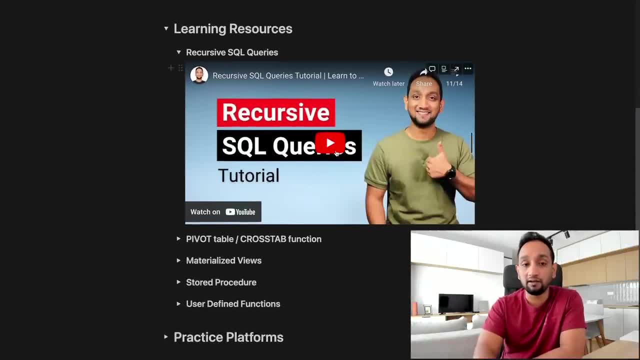 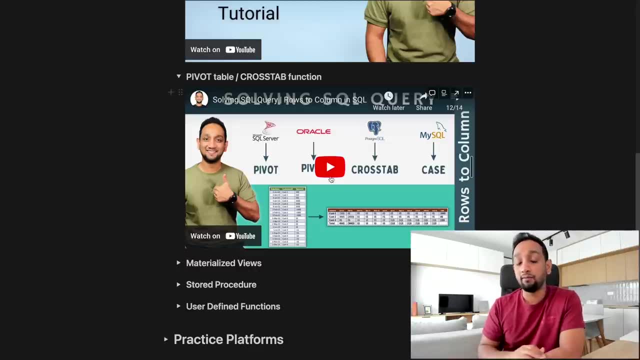 i have created a fantastic tutorial video on youtube. you could definitely check this out for pivot table or for crosstab. i have created this fantastic video where i have basically covered crosstab and basically converting rows to column in all these four major rdbms. in this video i 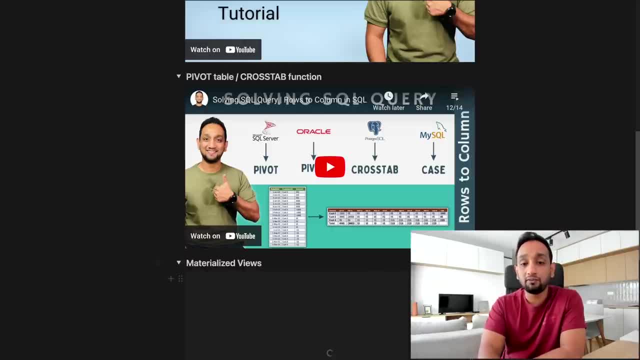 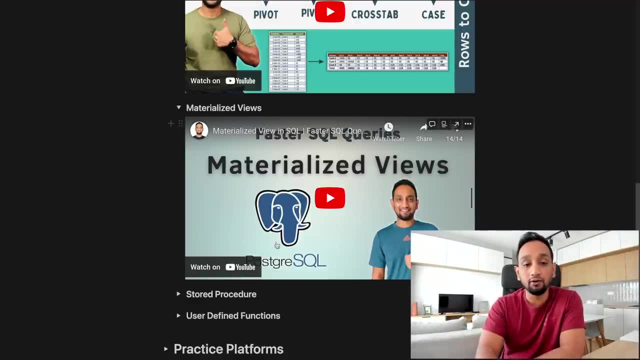 would definitely recommend you to check out this video for materialized view. again, i have created a tutorial on youtube which i would leave the link to in the description or in my blog, so definitely check that out for stored procedure. again, i have created a fantastic tutorial video. 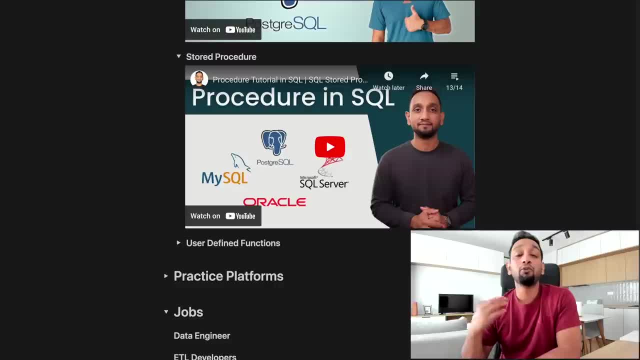 i would highly recommend you to check this out to get complete understanding of how to create and work with procedures in sql. okay, and finally, for user defined functions. i have not created a tutorial video, so i would recommend you to check out this blog that i will leave in the 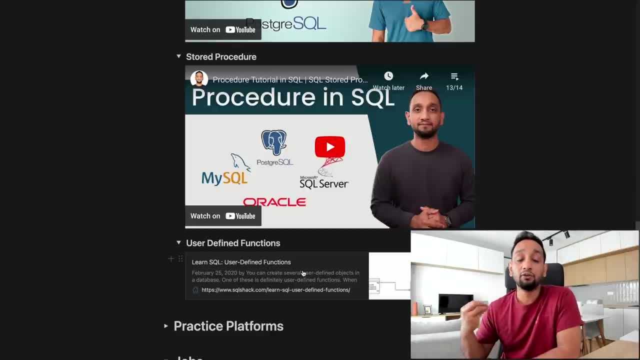 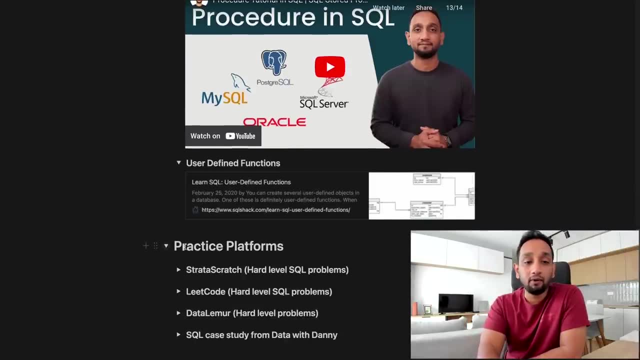 i'll leave the link in the description below. now, if you want me to make a tutorial video on user defined functions, definitely let me know in the comments below, so i can start working on that. now, when it comes to practice platforms again, the platforms that i would recommend is: 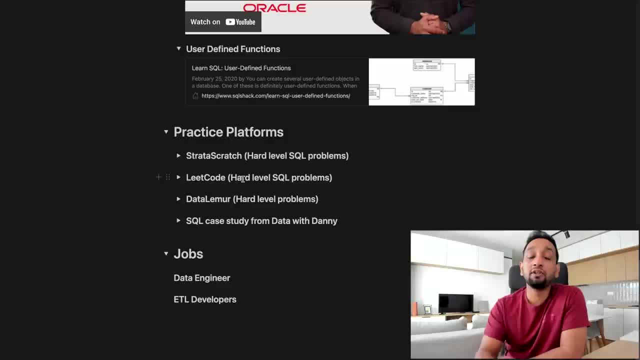 strataskratch, leetcode and datalemur. here you choose the hard level, hard difficulty level problems and try to solve it. okay, and when it comes to case study again, i would choose the same case study, data with danny. maybe you can decide between data with fd and data with dany. 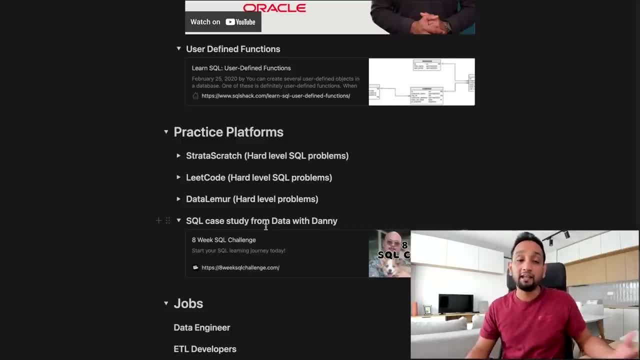 in as part of intermediate level of SQL. you didn't have to solve all the eight case studies. maybe couple of them would be sufficient, but when it comes to hard level of SQL you will. I think it's better you solve all the eight case studies and, again, jobs that you can target I have already. 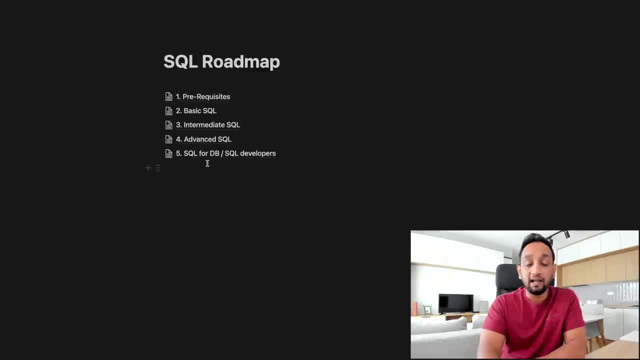 mentioned here. okay, so now let's look at the last section, that is, how much SQL should you learn if you are targeting to become a database developer or SQL developer? first of all, okay, jobs. you already know it's for database developer or SQL developer. the concepts that you will additionally need to. 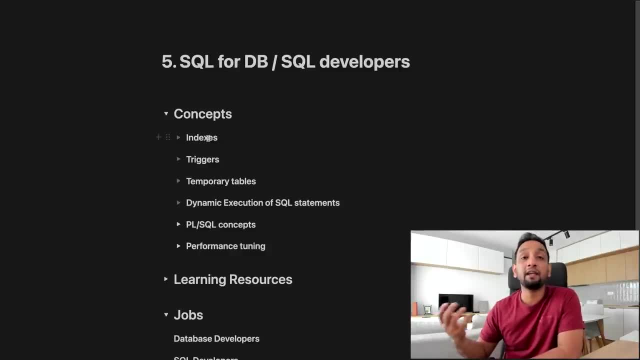 learn are. you need to know indexes? right, you need to know why indexes are useful- basically, how does it improve the performance of your query? and you need to know how to use the right index for your query. right, you should not be creating an index for every column, but you should know how, what is? 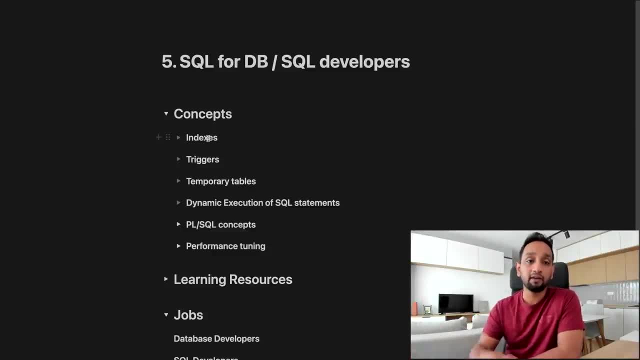 the right index you should create based on the query that you are frequently writing, right. you should then learn about triggers. you should learn about temporary tables. you should also know about how to dynamically execute an SQL statement right. and then you should also know about PL SQL concepts, because, as a database developer or an 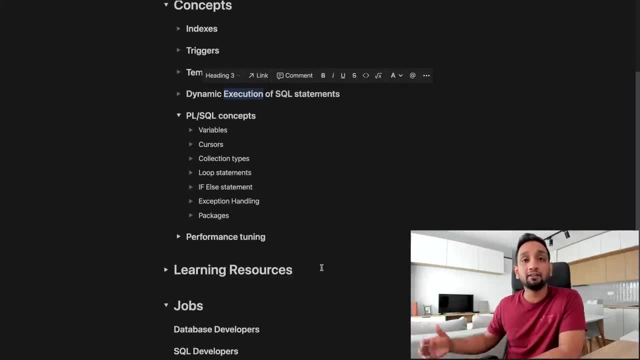 SQL developer, you would not only be writing SQL queries, but you would also be writing certain procedural language, maybe packages, procedures, user-defined functions, etc. and as part of that, you should be knowing what are variables, what are cursors, what are collection types or arrays, loop statements, if-else statements, exception handling and packages. right, and after all of this, one very 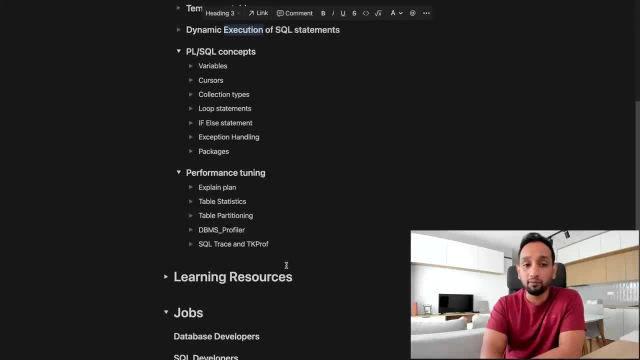 important thing that you will need to learn is performance tuning. now, when it comes to performance tuning, you will mainly need to know what is explained plan, how to basically read and explain plan. you need to understand that. you need to know how does stable statistics basically help in improving the performance? you need to know about table partitioning and then, finally, these: 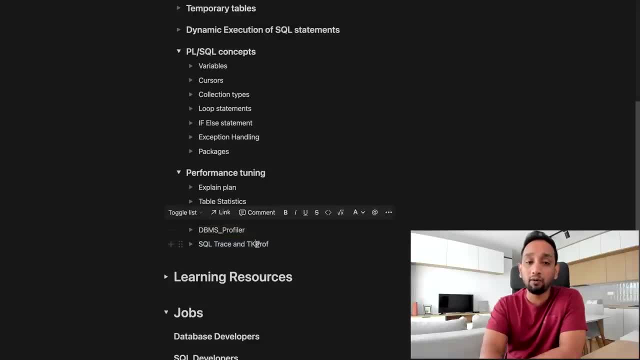 three concepts in DBMS: profiler, SQL trace and TK prof. these are the concepts specific to Oracle, but these are mainly used if you want to track the performance of your procedures or your SQL queries, and I'm sure there are alternate ways to this in other RDBMS processes, but I think it is important to 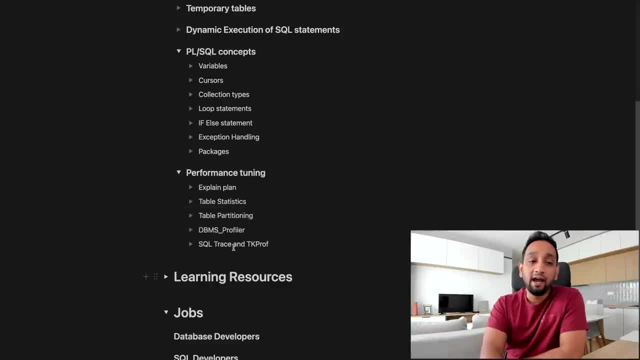 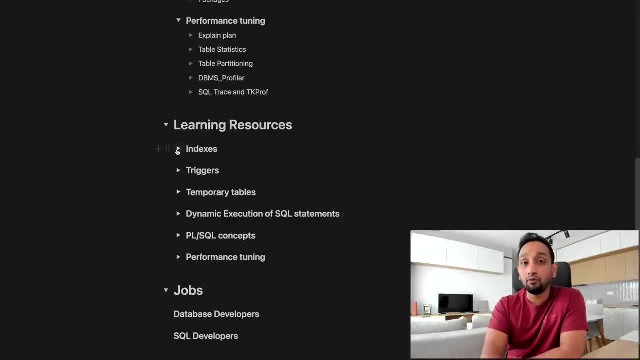 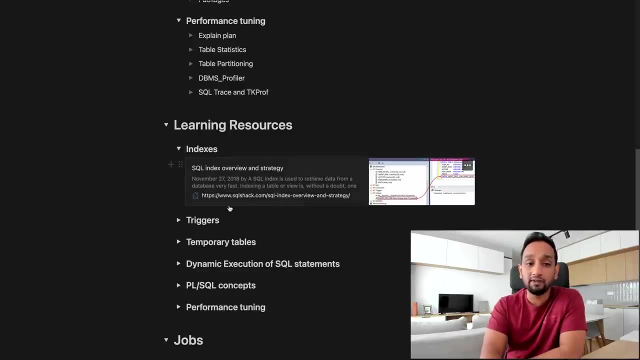 know these concepts okay and as part of learning resources for indexes. now I have not created a tutorial video on any of these concepts, but I have found some very useful resources online, so I'm going to mention that. for indexes, I have this blog, which I found. I'll leave that, and similarly for